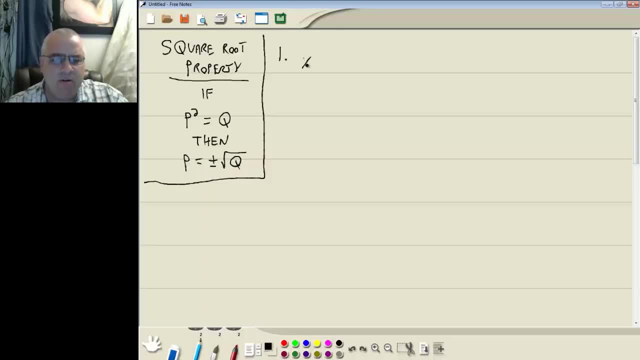 We got x squared is equal to 25.. Now this property says the entire left side has to be squared. As I look at this problem right here, I see the entire left side, So we can apply our square root property directly. So we drop our squared and we put a plus or minus square root around the other side. 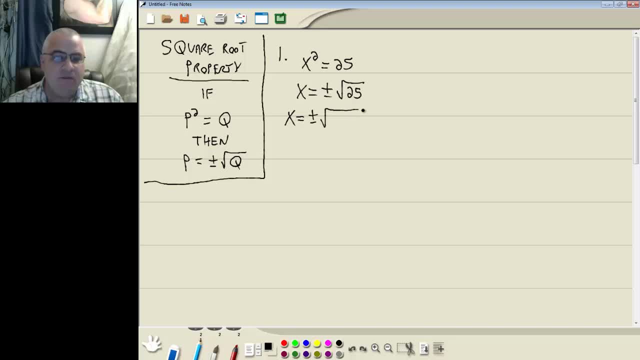 Now, always, you should simplify your radicals before you go on. 25 is 5 times 5, and remember, with square roots we're looking for pairs of something. Here's a pair of 5, so this pair of 5 is going to come out in front as a single 5.. 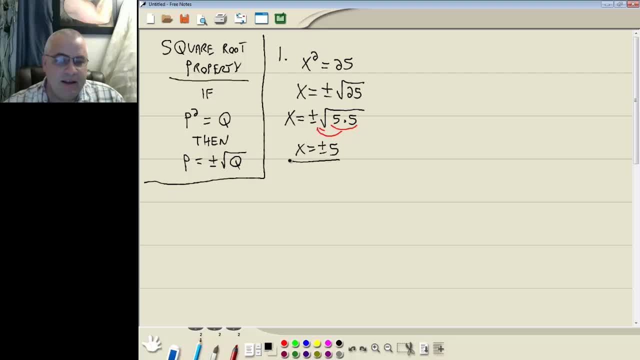 So we got x is equal to plus or minus 5.. Now that's our answer. If you're not familiar with this notation, what that means is it means we got x is equal to negative 5, and we got x is equal to positive 5.. 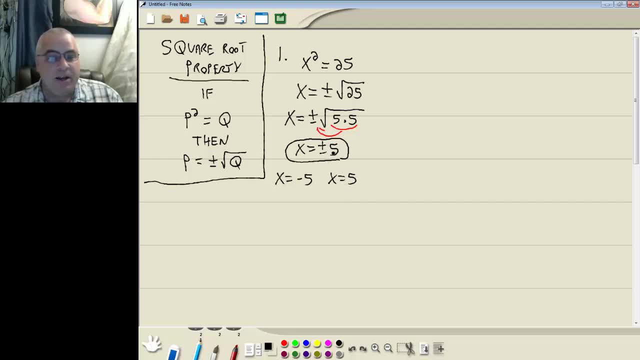 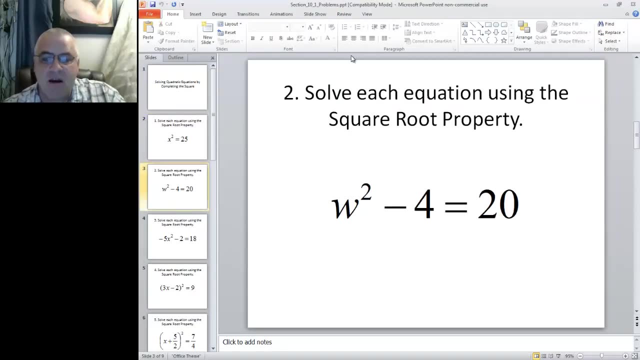 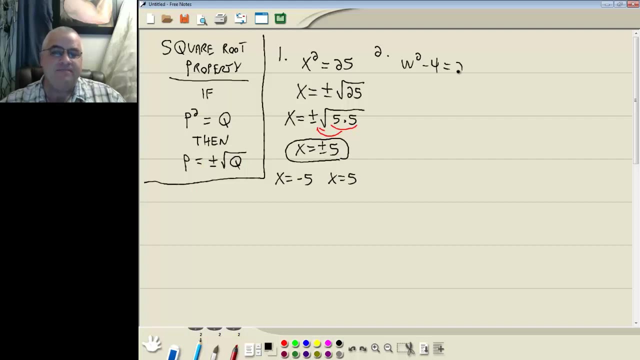 So we got two answers. Typically, a simplified form means you leave it with what I circled. Take a look at our second example. We got w squared minus 4 is equal to 20.. Notice, on this particular problem, The entire left side isn't squared. 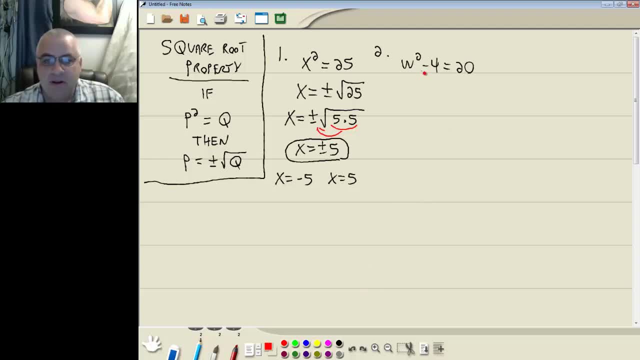 So our first step is to get the part that's squared by itself. So I'm going to take this negative 4 and move it to the right side. So we got w. squared is equal to 20 plus 4.. Remember you move anything across your equals, your sign changes. 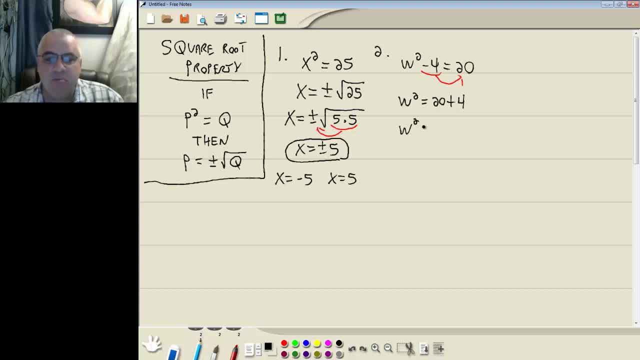 So negative 4 becomes a positive 4.. Add those together, 20 plus 4, is 24.. Now the entire left side is squared. So that's all. our square root property says: You got something squared equal to something else. So we drop our squared and we put a plus or minus square root around the other side. 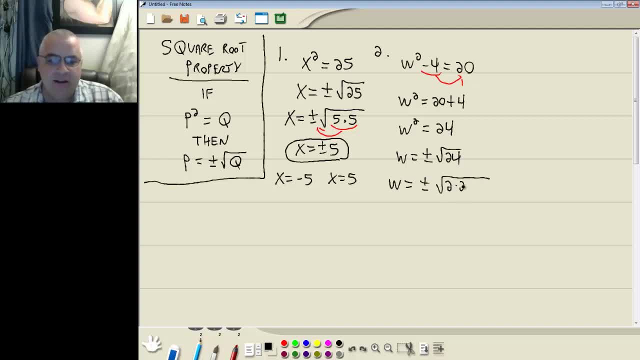 Always simplify your radicals. 24 is 2, 4,, 8 times 3.. Remember the square root. we're looking for pairs or something. Here's a pair of 2's, So this pair of 2's is going to come out in front as a single 2.. 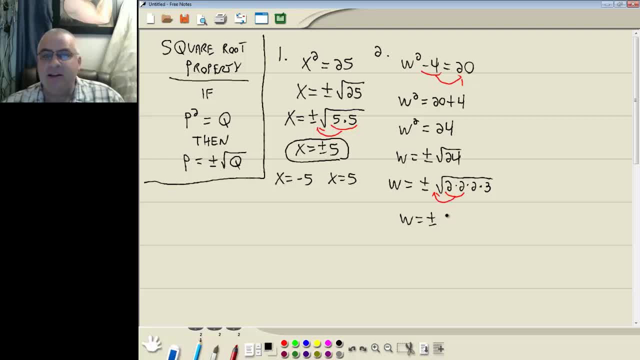 So we got: w is equal to plus or minus 2.. And we got a 2 and 3 left inside, and again we have to have pairs of them to bring them out. So all we do is multiply those together. 2 times 3 is 6.. 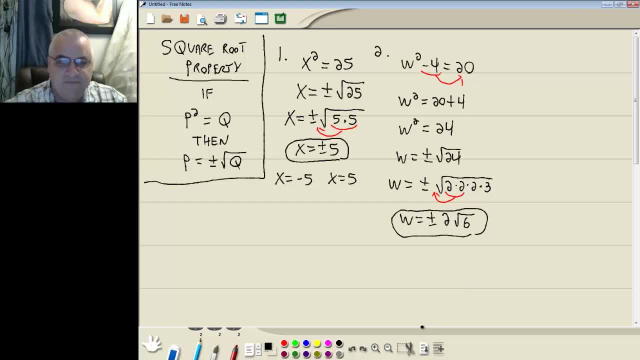 So our answer is: w is equal to plus or minus 2 squared over 6.. Let's take a look at this problem: Negative 5x squared minus 2 is equal to 18.. Obviously, 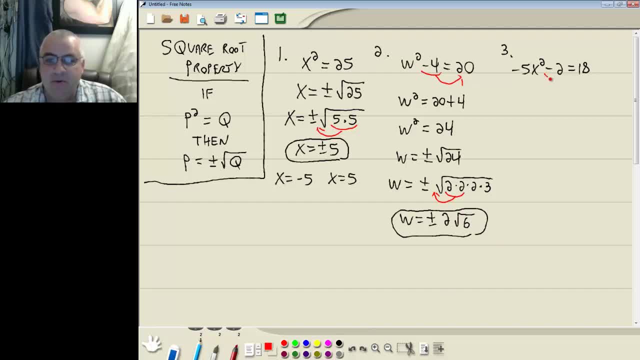 2 squared. so let's work at getting the part squared by itself. Take the negative 2 and move it to the right side. Remember, when you take anything across, your equal sign changes. So negative 2 becomes a positive 2. then 18 plus 2 gives 20.. 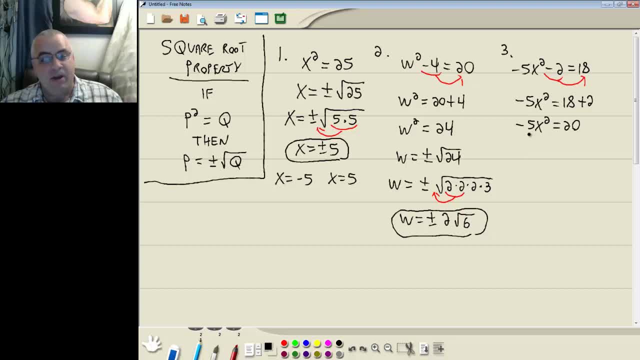 Now the only thing squared is the x. The negative 5 isn't squared, so we still don't have it in the right form. yet The entire left side has to be squared- squared. Well, to get the part to square by itself, we'll divide both sides by. 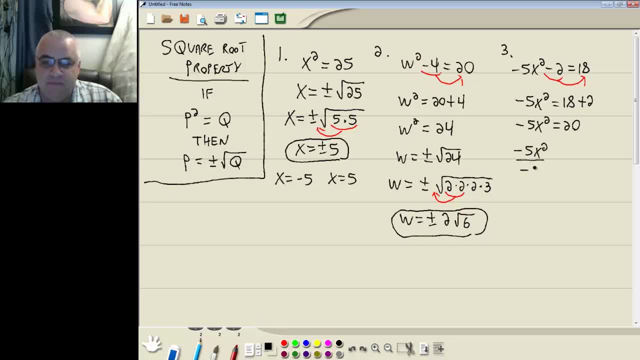 negative 5.. Do that, we get x squared, and 20 divided by negative 5 gives us a negative 4.. And now it is in the right form. We got something squared equal to something else. Square root property says we drop our squared and we put a plus or minus. 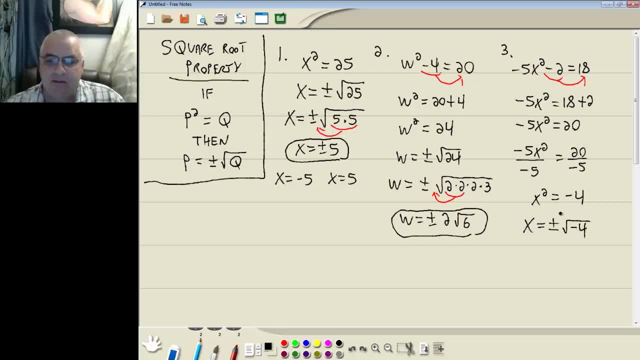 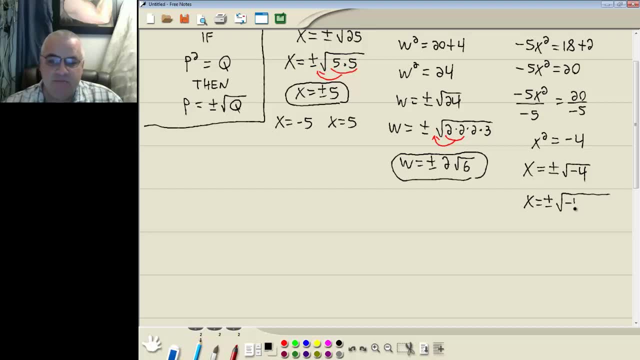 square root around the other side. Now we want to simplify our radical now Negative 4, that's negative 1 times 2 times 2.. If you remember, from complex numbers a negative 1 inside of a square root comes out as an i, and here we got a. 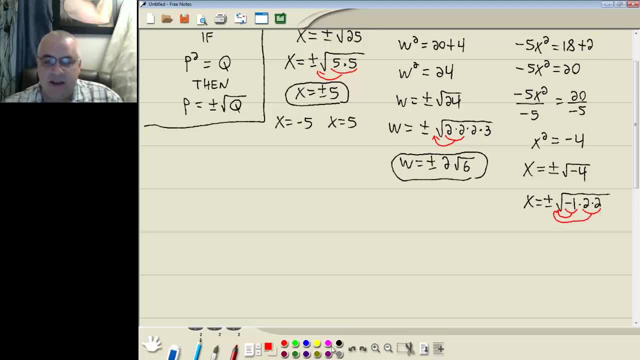 pair of twos. A pair of twos is going to come out in front as a single 2.. So we're going to have: x is equal to plus or minus 2i, And that's your answer. Okay, let's look at this one. We have 3x minus 2 squared equals 2, 9.. Now right. 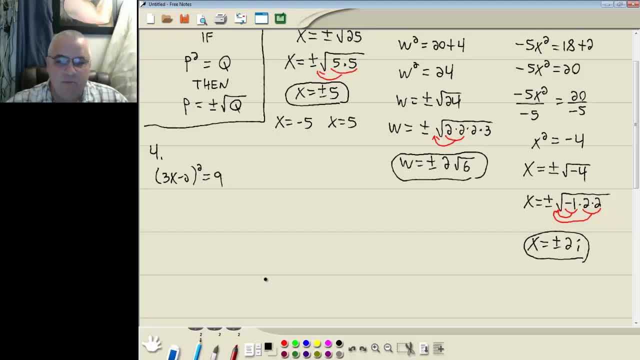 away. this is already in the right form. we got something squared equal to something else. So square root property says we drop our squared and we put a plus or minus square root around x square root and drop our squared on the other side. now, always, you should simplify radicals before you go on so in. 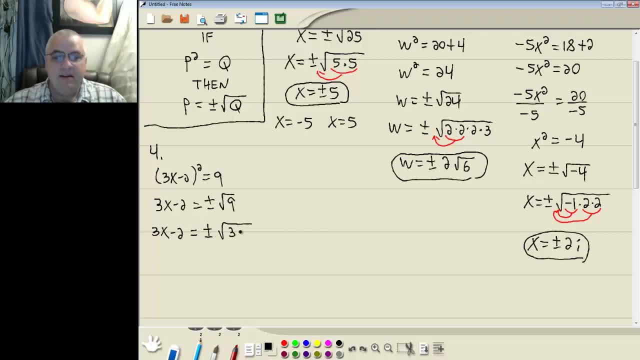 this case we got 9, which is 3 times 3, and remember the square root. we're looking for a pair of something's, so here we got pair of threes. they're going to come out in front as a single 3, so we've got 3x minus 2 is equal to plus, or? 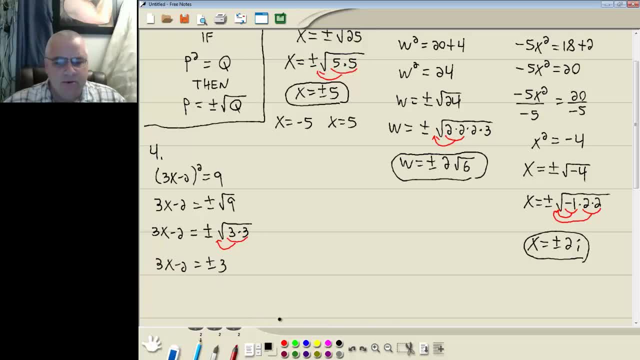 minus 3. now I took everything out of the radicals. the radical just disappears. now our goal is to get the X by itself, so I'm gonna take this negative 2 and move it to the right side. so we got 3x is equal to 2 plus or minus 3. and then I 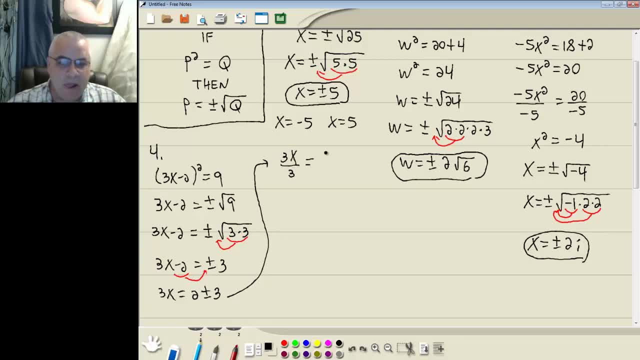 want to divide both sides by 3 in order to get the X by itself and we got. X is equal to 2 plus or minus 3 over 3. sometimes it's beneficial um to split it apart into the plus side and the minus side. 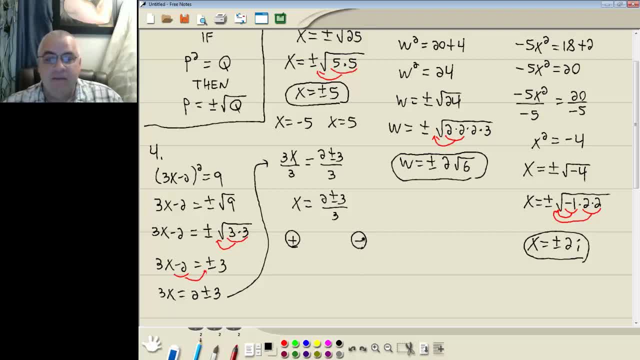 When? when is it beneficial to do this? When your, when your radical disappears And it looks like. maybe you can do a little bit more simplifying. Now our first problem here: a radical disappeared. we got plus or minus five, but obviously putting those into two separate pieces doesn't simplify. 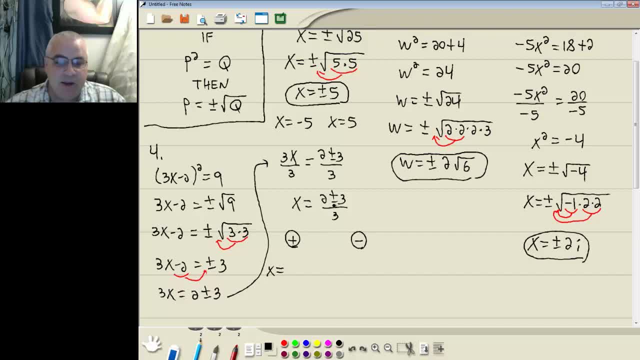 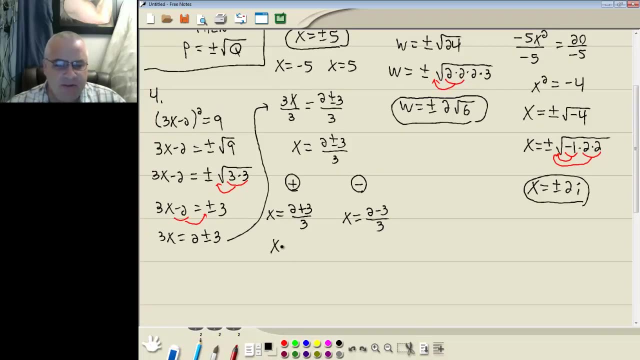 But let's see what happens in this problem. What that plus or minus means is we're going to have x is equal to two plus three over three, and we'll have x is equal to two minus three over three. Now see, after I split those up into two separate pieces, I can simplify it. 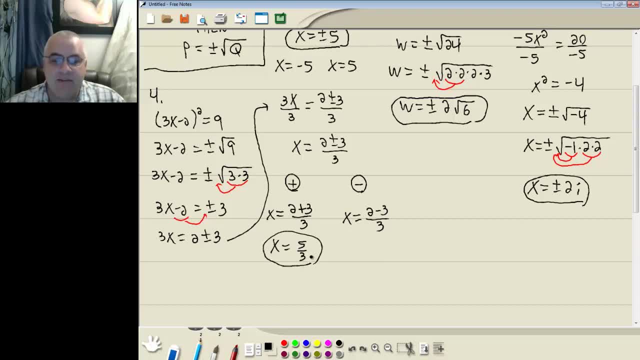 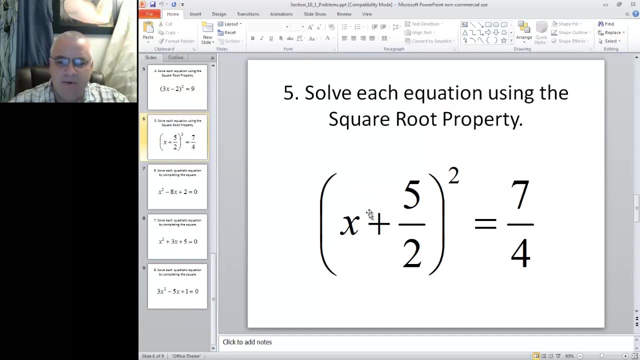 Two plus three is five, so we got x is equal to five thirds. And over here we got two minus three, which is negative one. so we got x is equal to negative one third. And those are our two answers. Let's take a look at one more and then we'll take a look at completing the square. 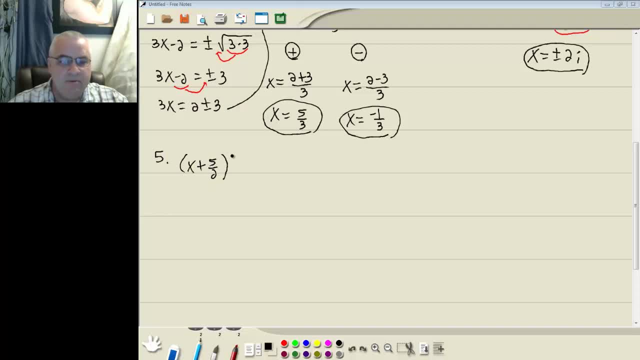 So we got x plus five halves. squared is equal to seven fourths. Now again, all the square root property says is if you got something squared equal to something else, then you can apply it. So we'll apply it here. We'll drop our squared. 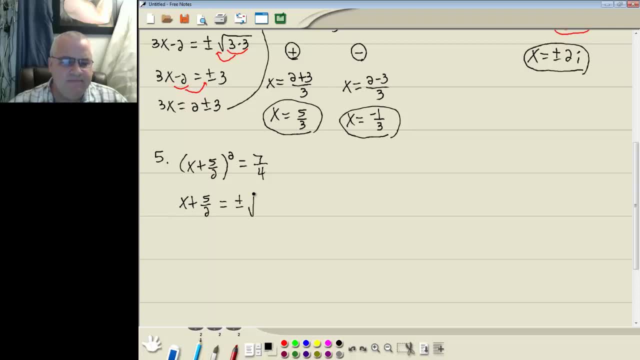 and we'll put a plus or minus square root around the other side. Well, we got a problem here. Remember when we were working with radicals? we said: you can't have a fraction inside of a radical. We've got a property that says: if you 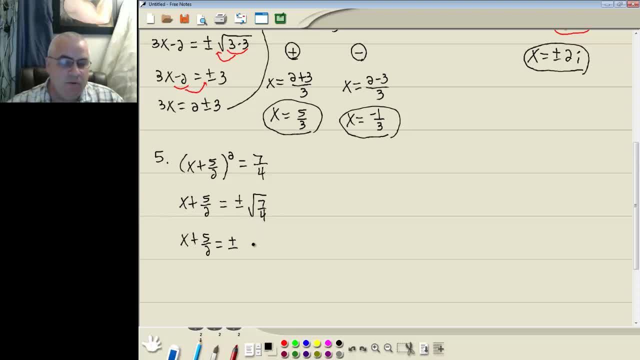 got a fraction inside of a radical. you can put a radical around the top, radical around the bottom. So we're going to have square root of seven over square root of four. Now that creates another issue. We also said you can't have a radical in the denominator, But in this case it's going to 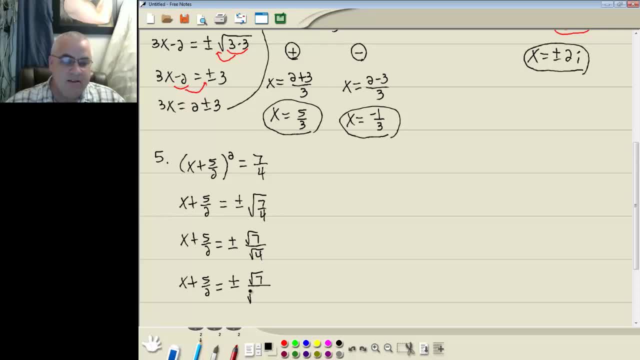 work out nice. Square root of four Four is two times two, So we can simplify this radical. Remember: with square root we're looking for pairs of something. Here's a pair of twos. They're going to come out in front. 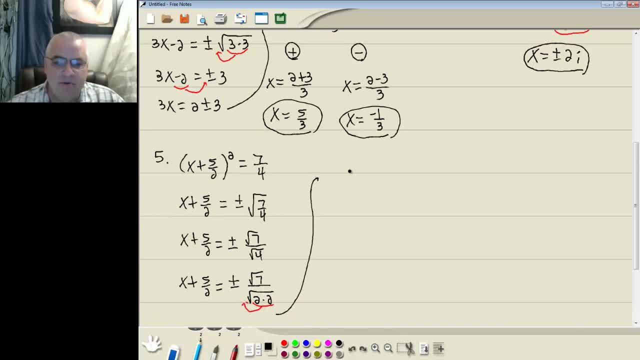 as a single two. So we got x plus five halves is equal to plus or minus square root of seven over two. Now our goal is to get the x by itself. So I'm going to take this five halves and move it over And we got x is equal to negative five halves plus or minus square root of seven over two. 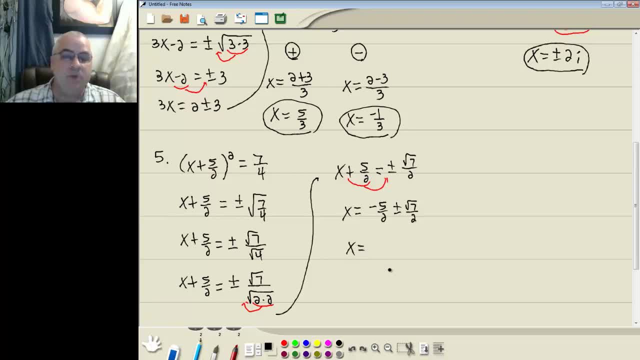 Typically simplified form, unless you have an imaginary part, an i. typically simplified form means merge into a single fraction, And especially these are so easy because they got the same denominator, So it's going to become negative. five plus or minus square root of seven all over two. 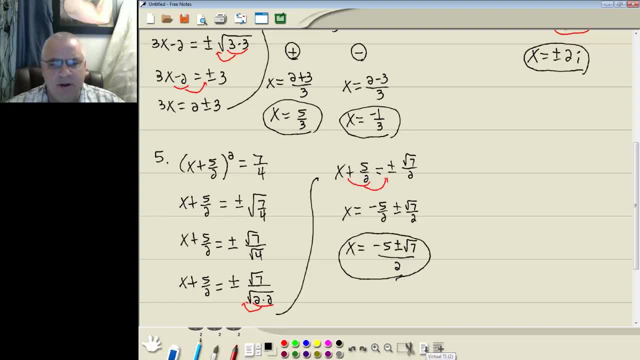 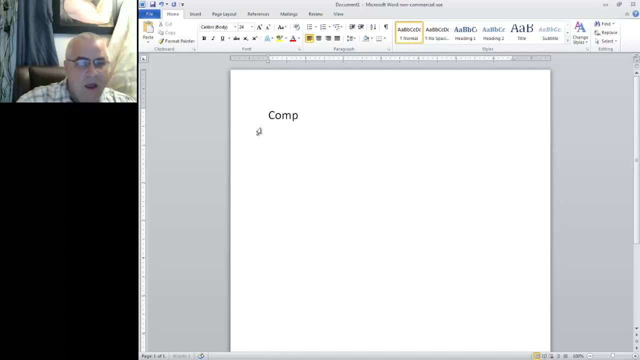 And that would be our answer. Well, let's take a look at completing the square now. Okay, completing the square. Excuse me. Step one: We want to divide everything, all the terms, by the number in front of the x squared. 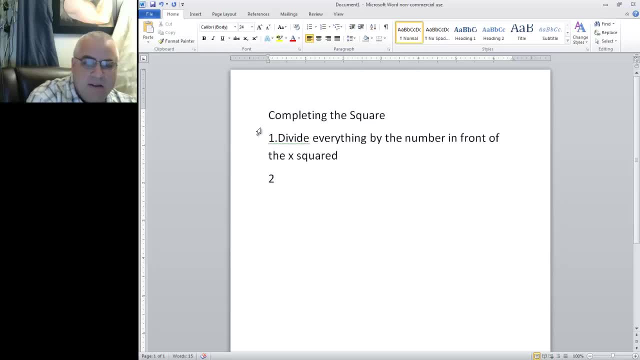 Step two is we want to take the number, the constant term, to the right side. Step three: take the number in front of the x coefficient, multiply it by one, half, square it and then add to both sides. Step four: back to the left side. 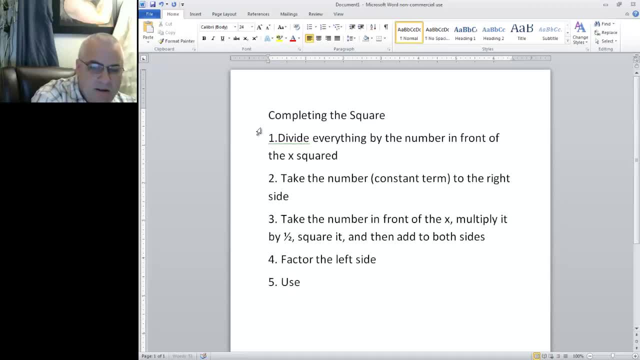 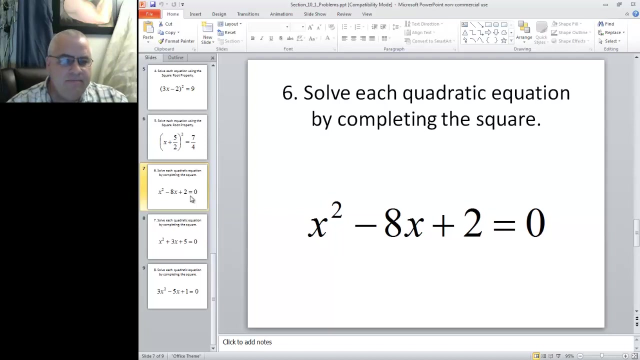 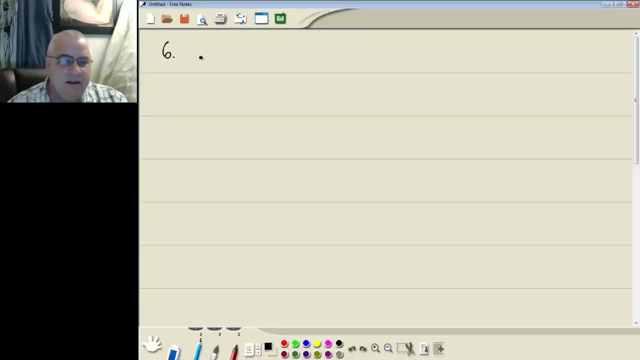 And step five use the square root property to solve for x. Okay, let's take a look at some problems dealing with this. and it goes in. this is the easiest type and we'll look at the medium difficulty and then look at the hardest type. so we got x squared minus 8x plus 2 is equal. 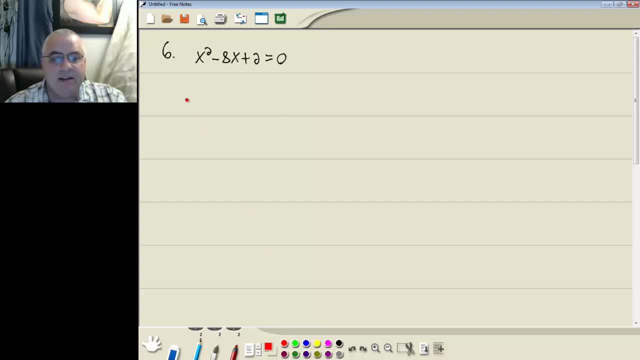 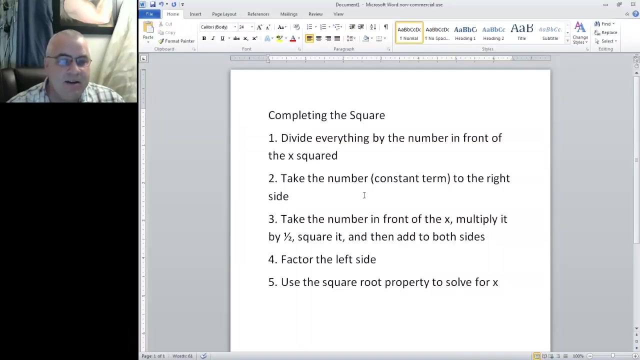 to 0. step 1: divide everything by the number in front of the x squared. we don't have a number in front of our x squared, so we don't do step 1 here. step 2: take the number or constant term to the right side. so I'm gonna take this. 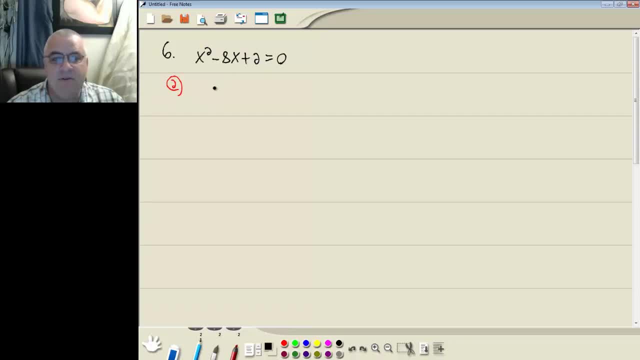 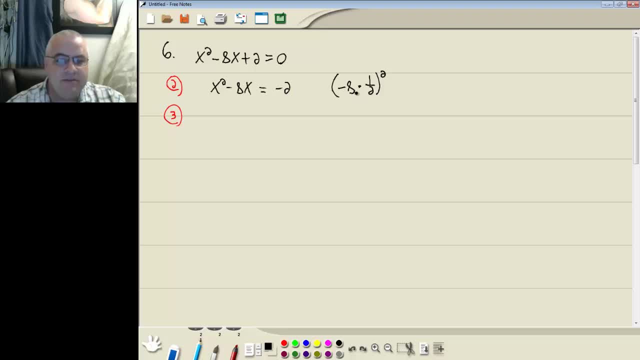 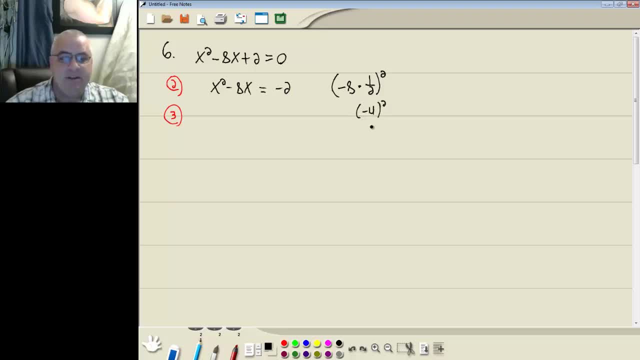 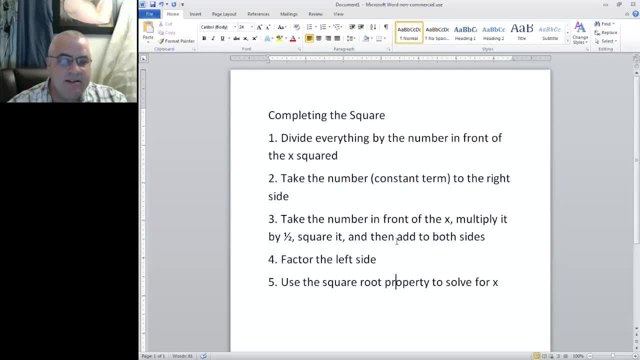 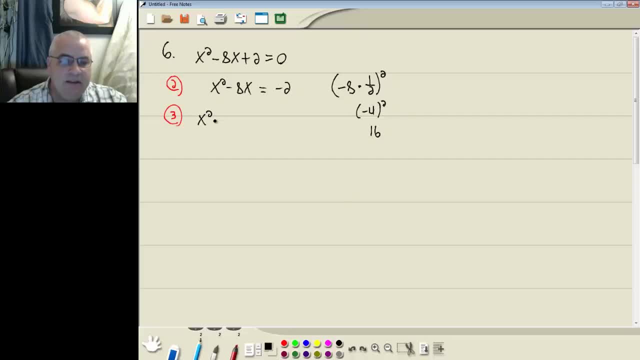 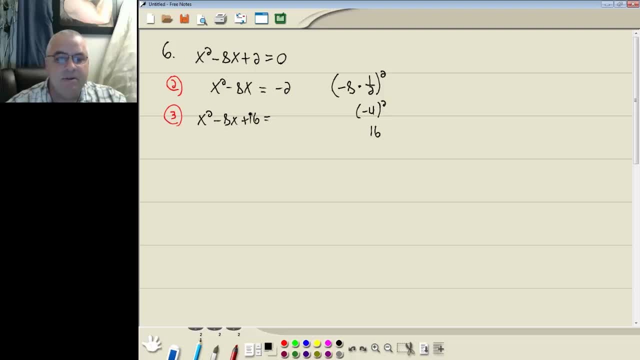 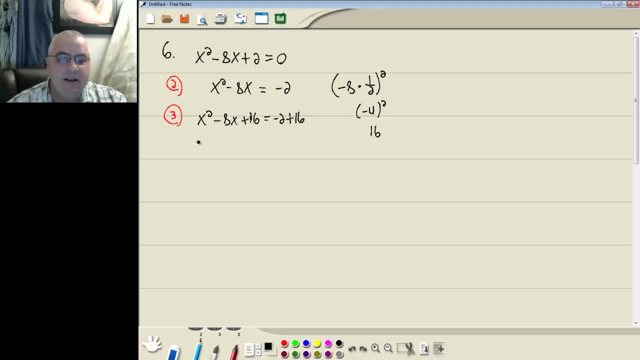 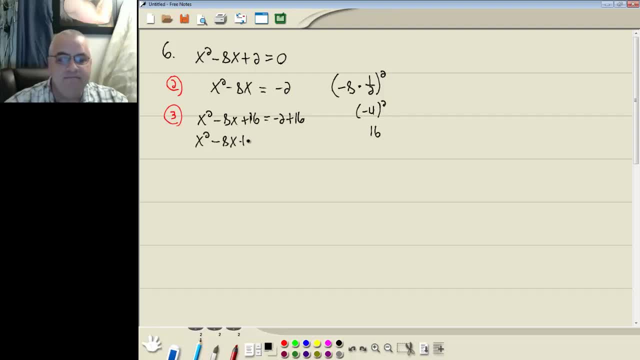 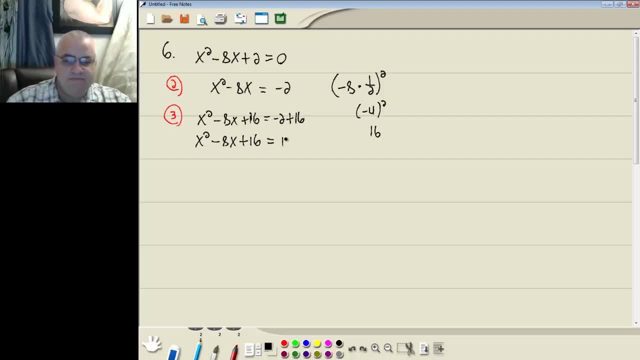 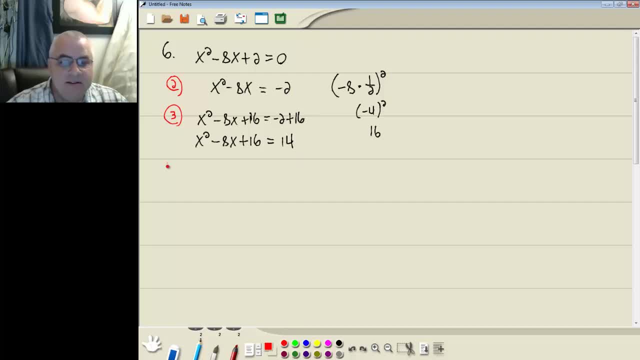 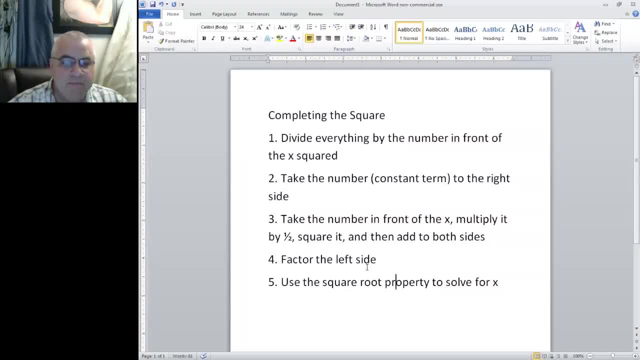 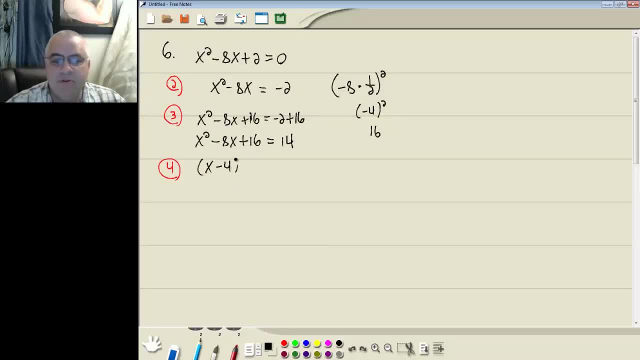 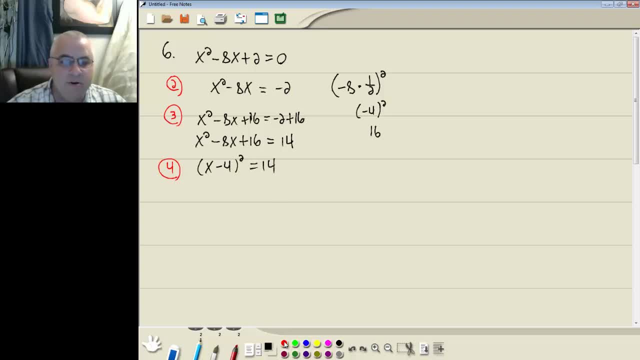 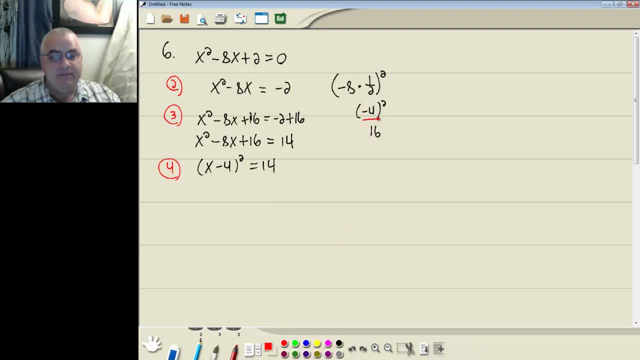 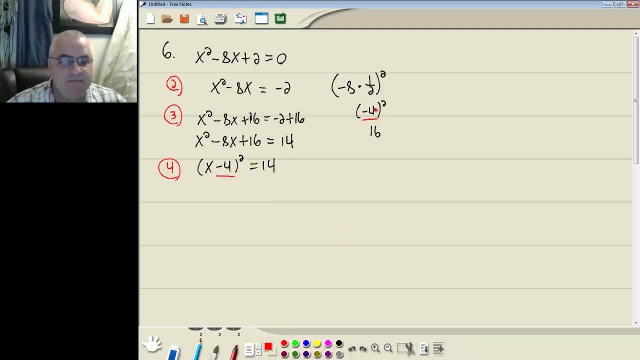 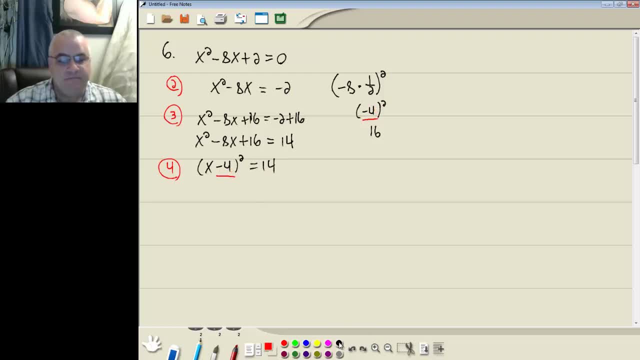 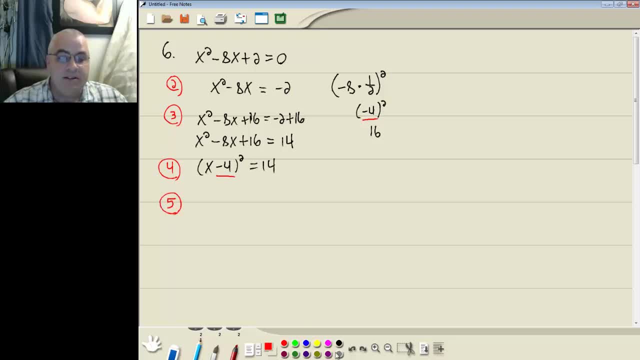 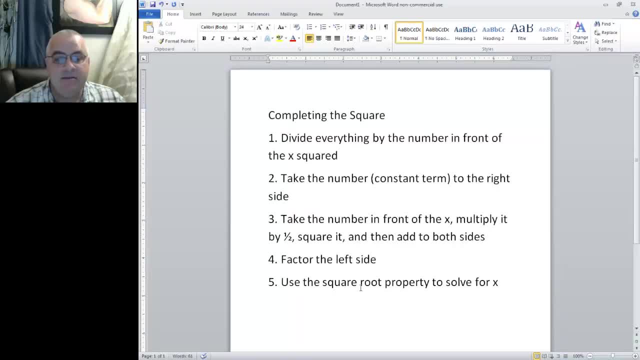 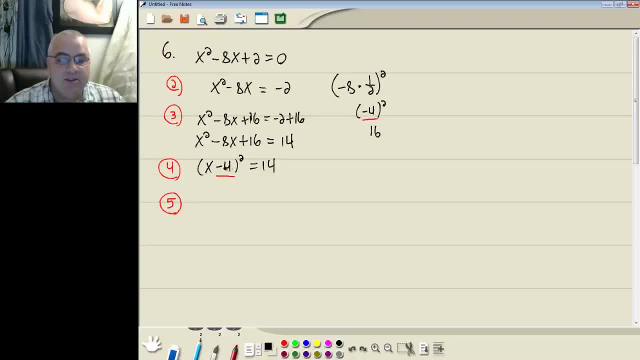 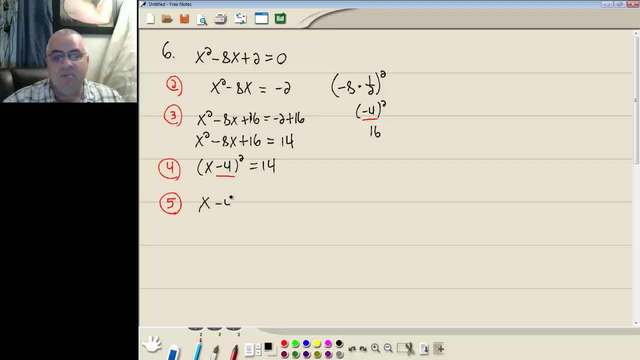 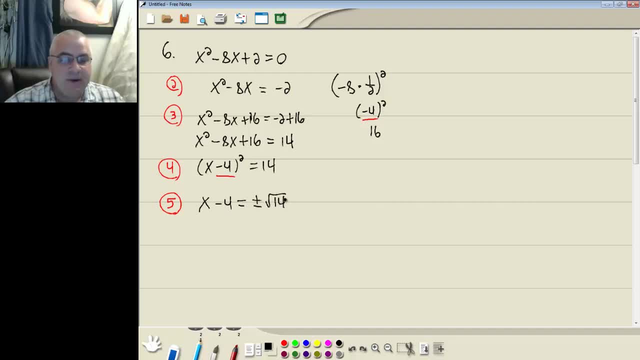 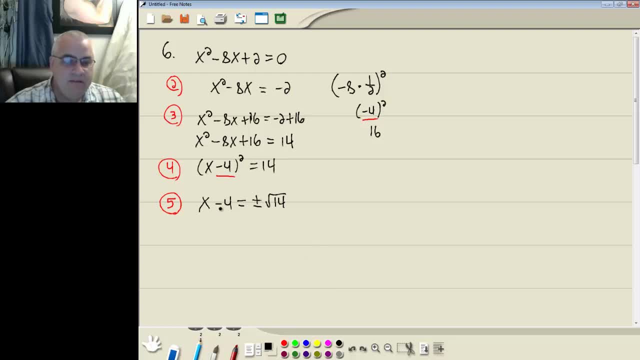 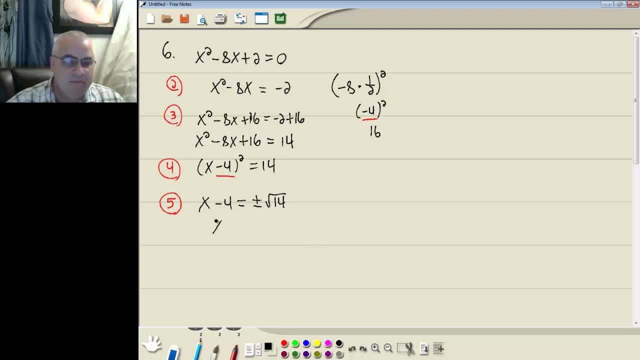 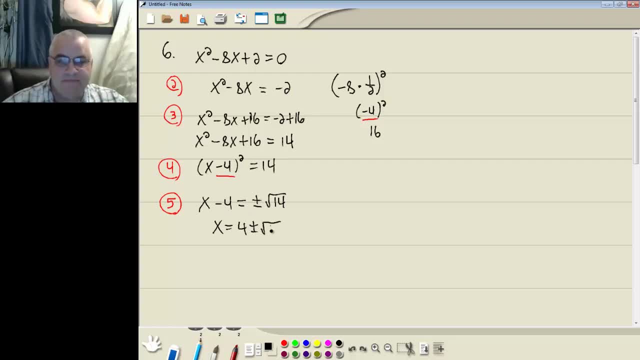 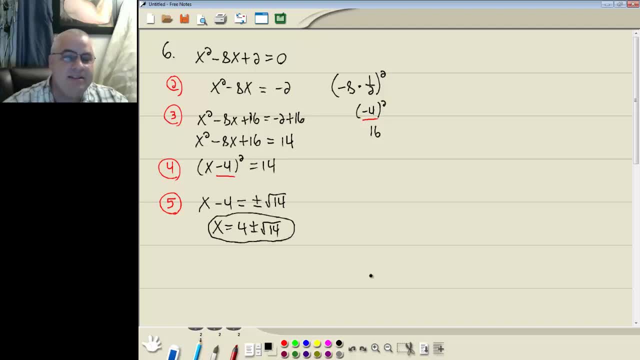 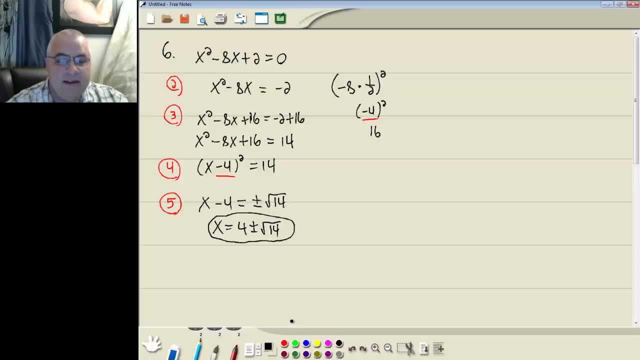 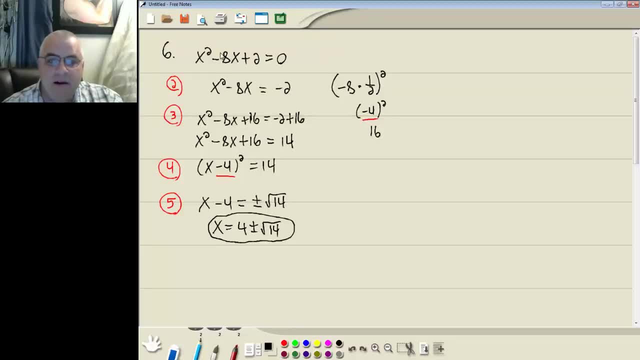 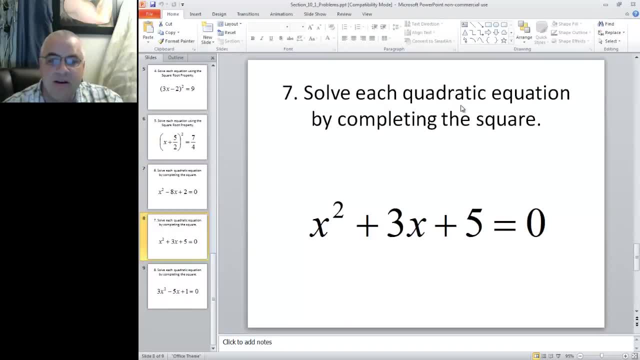 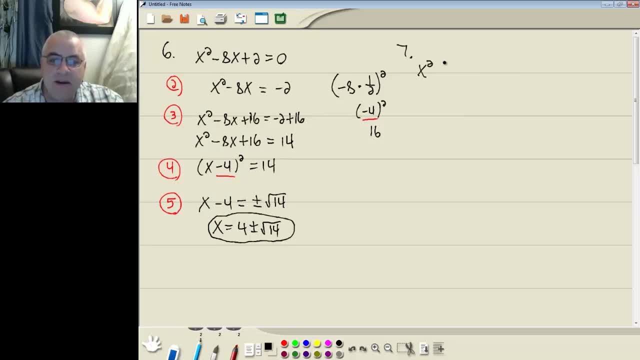 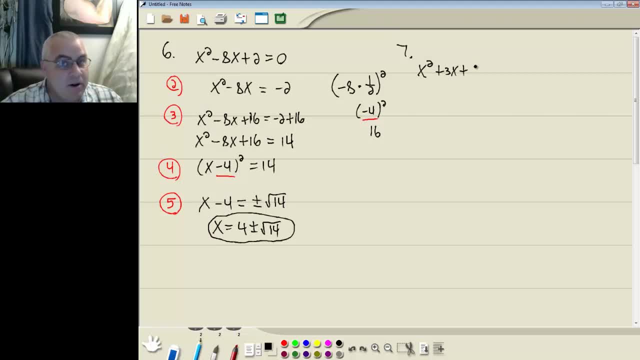 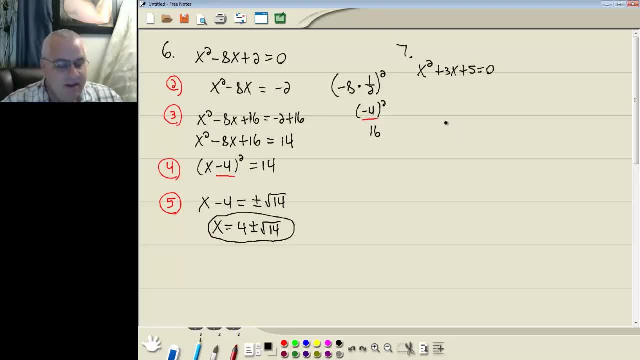 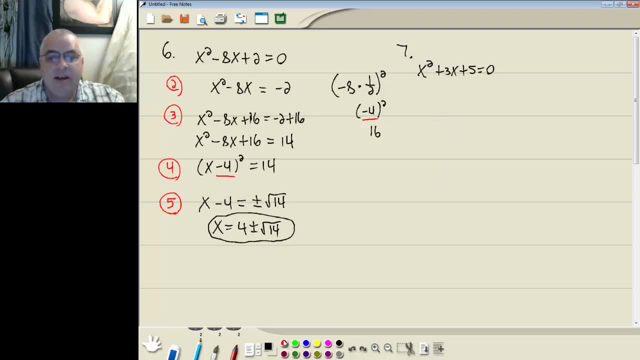 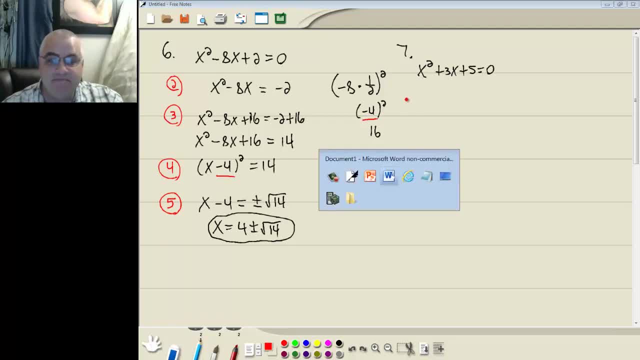 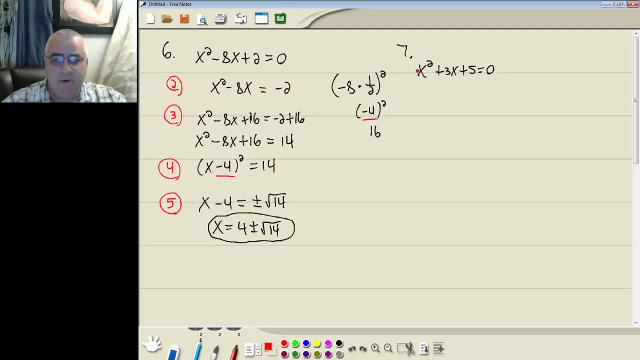 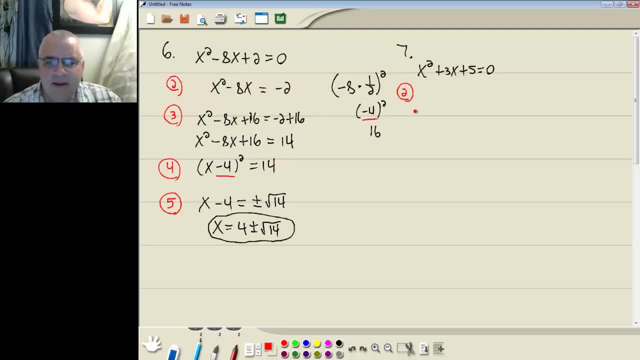 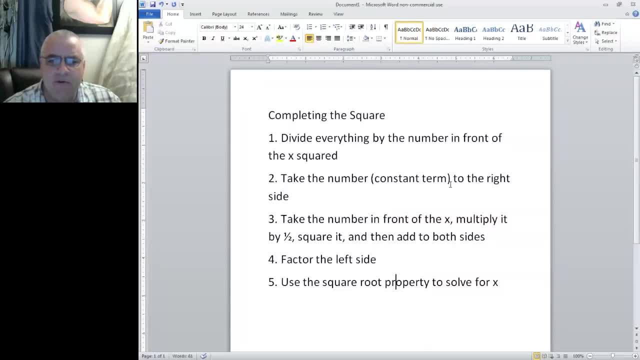 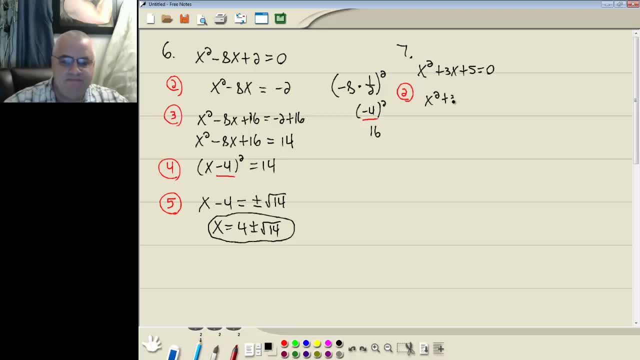 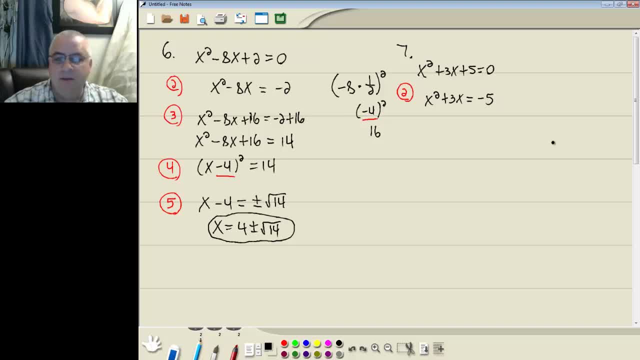 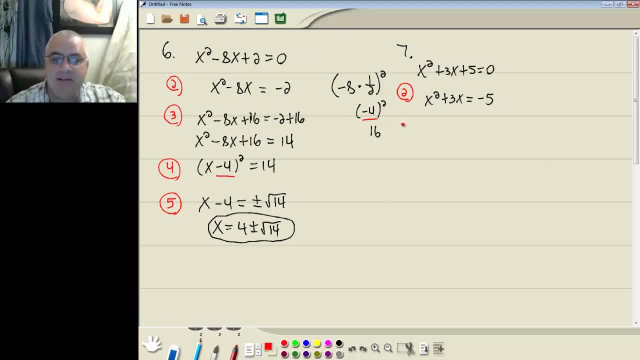 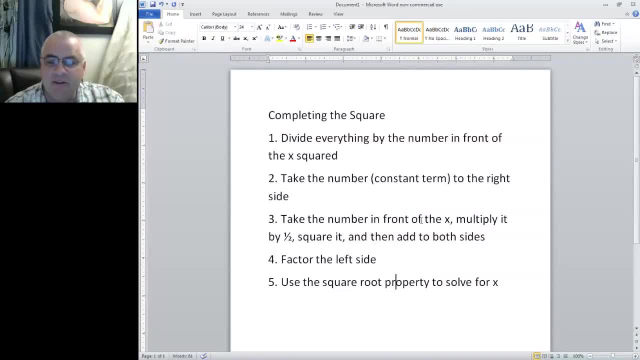 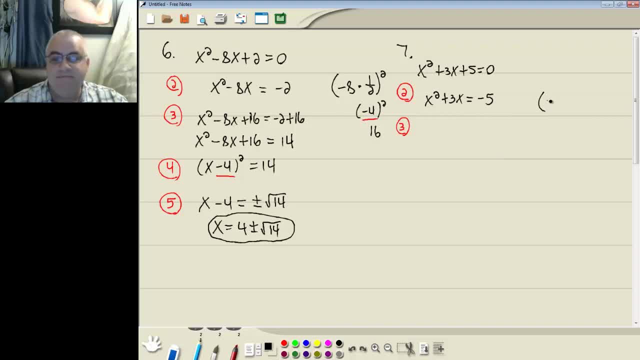 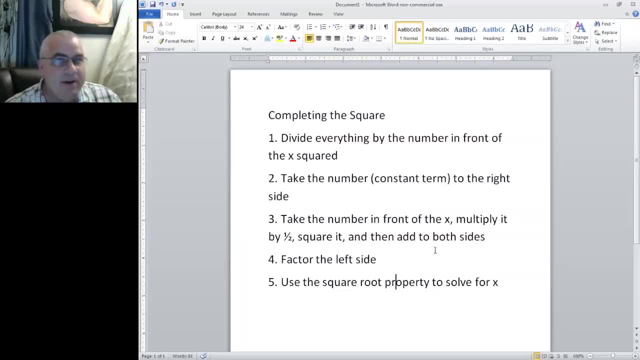 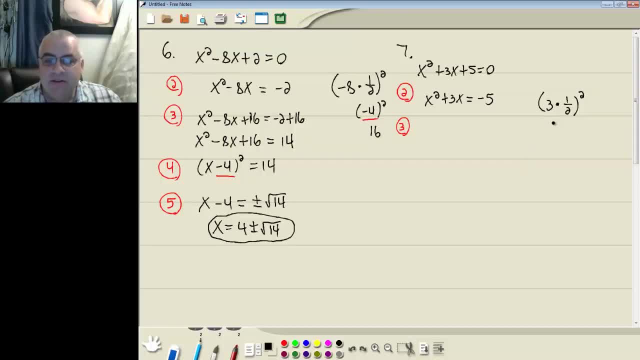 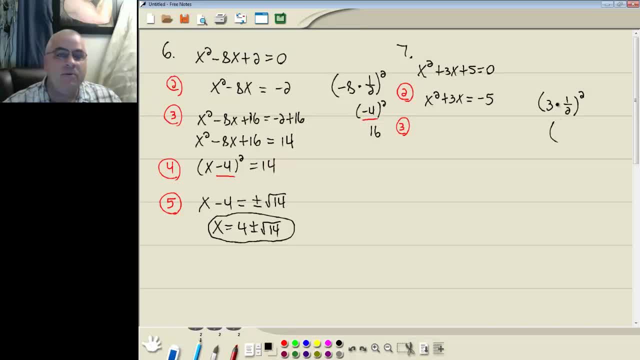 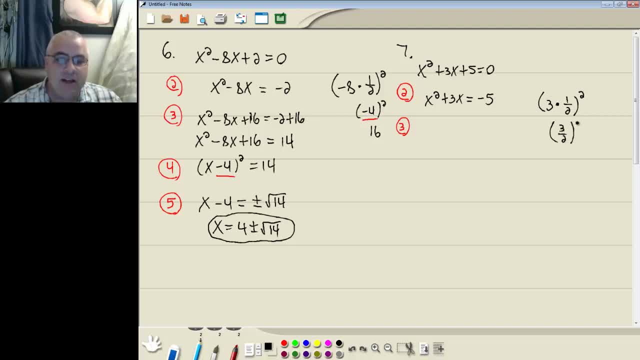 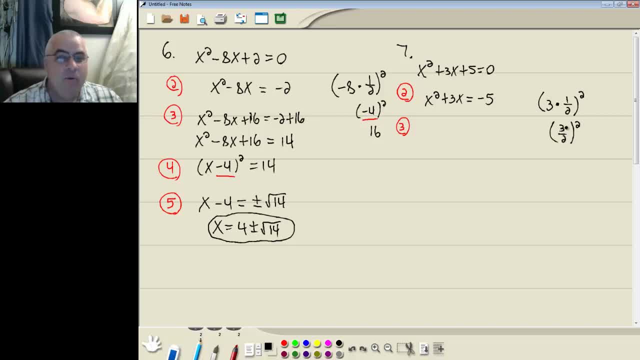 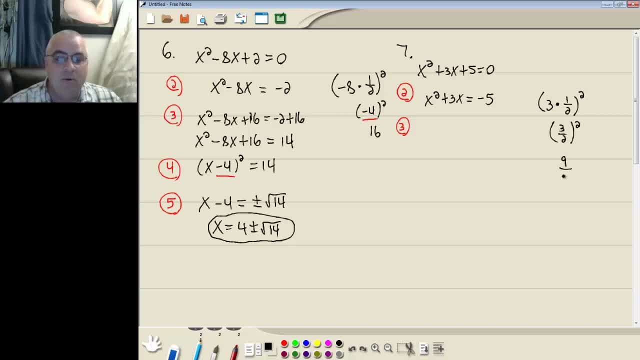 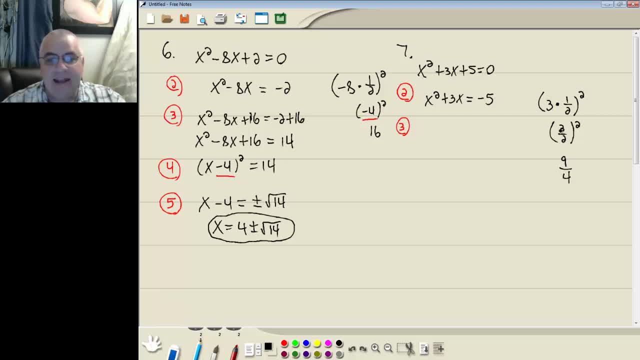 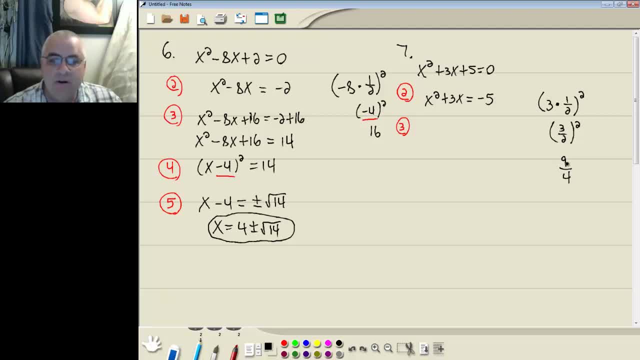 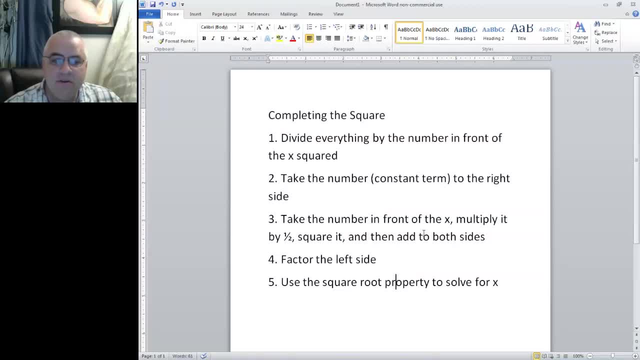 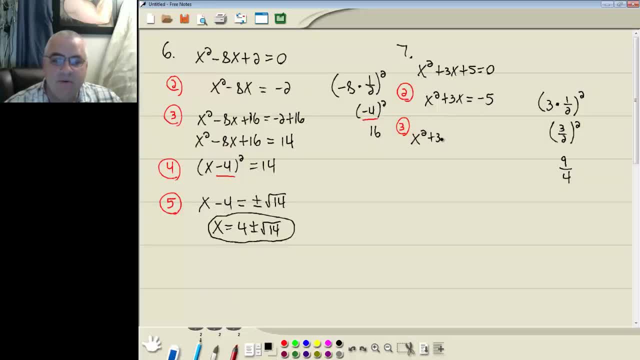 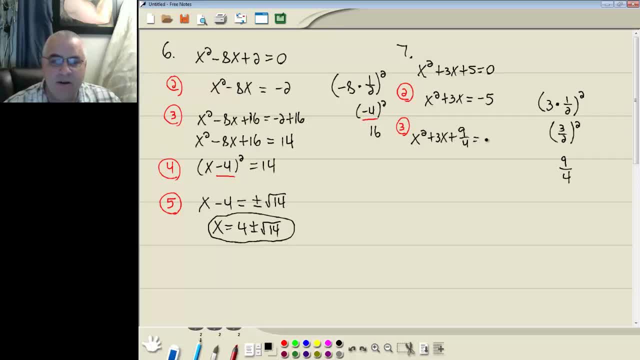 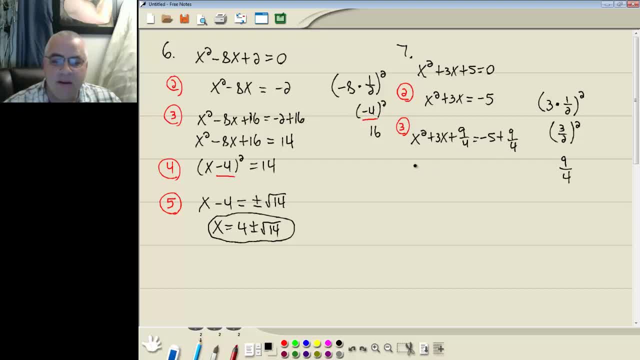 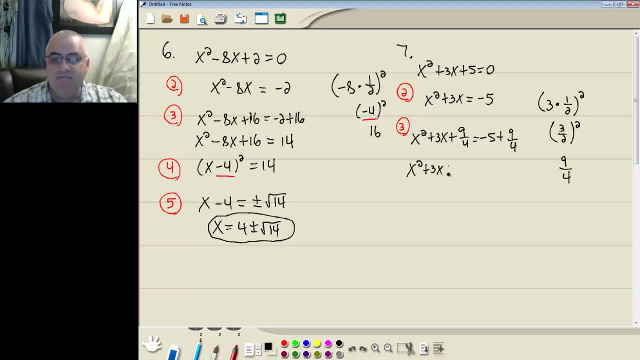 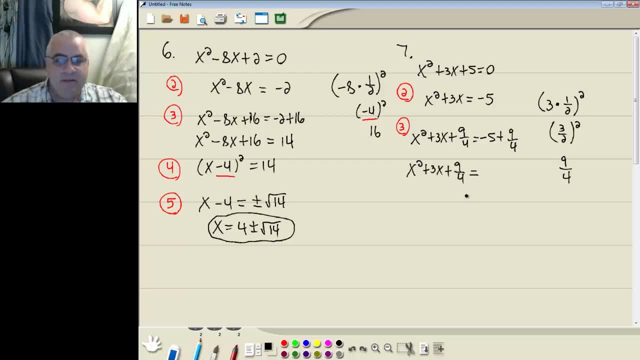 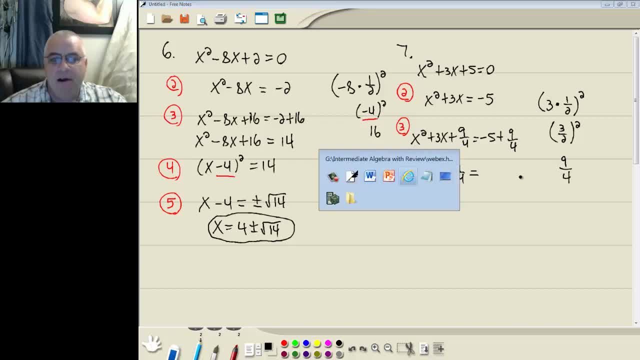 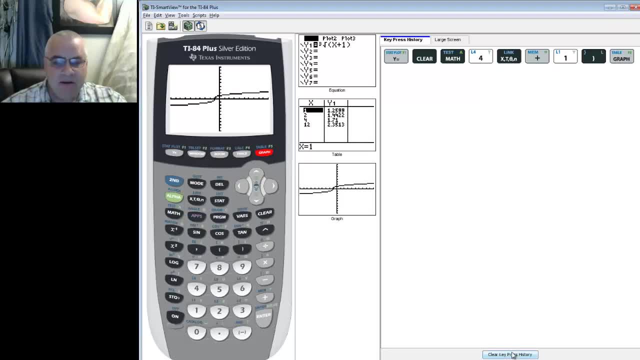 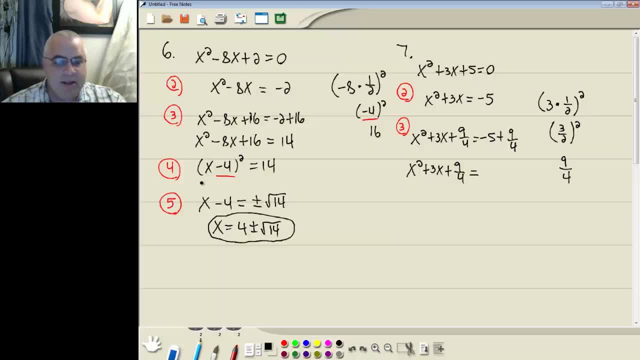 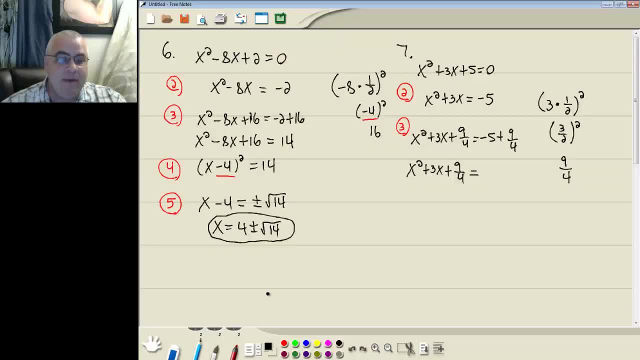 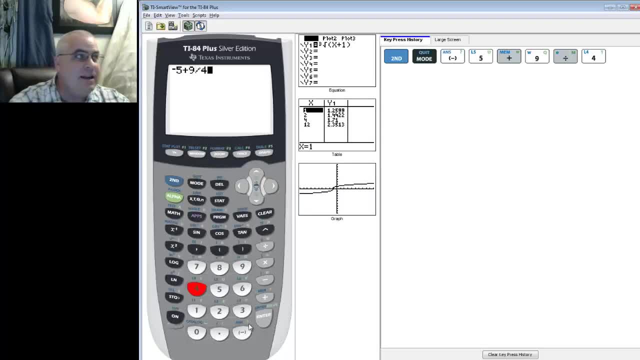 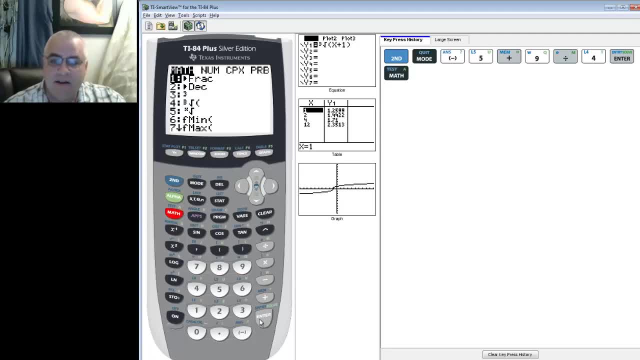 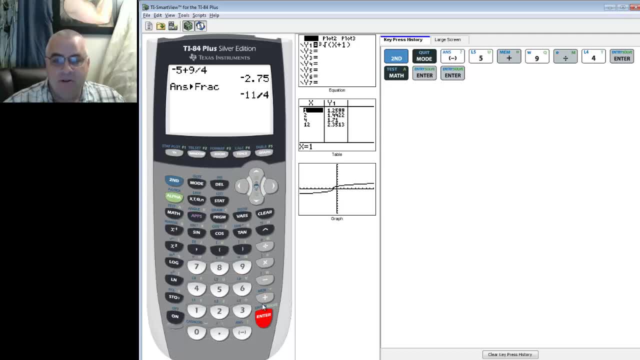 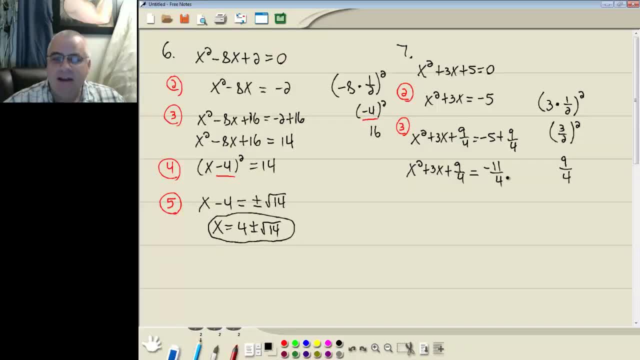 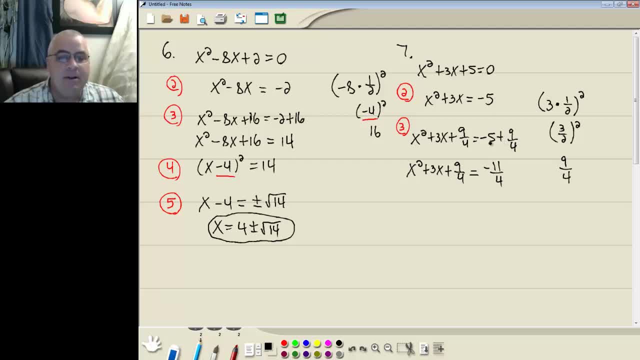 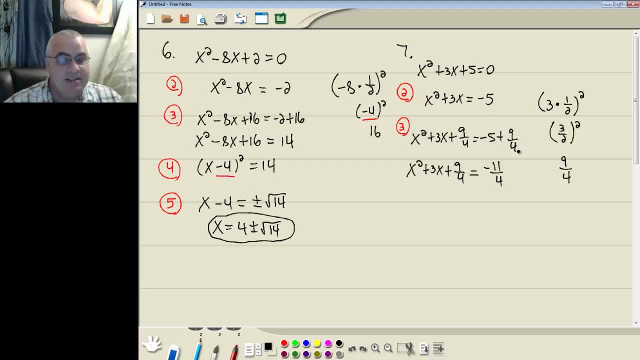 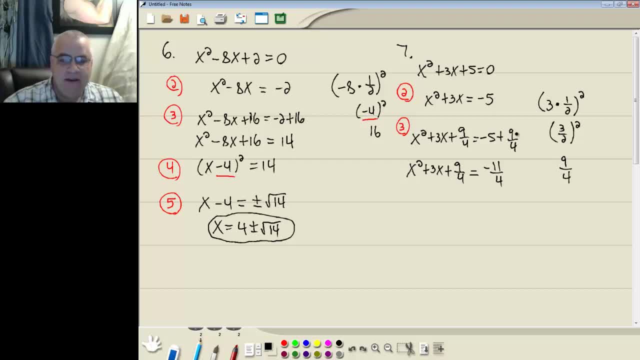 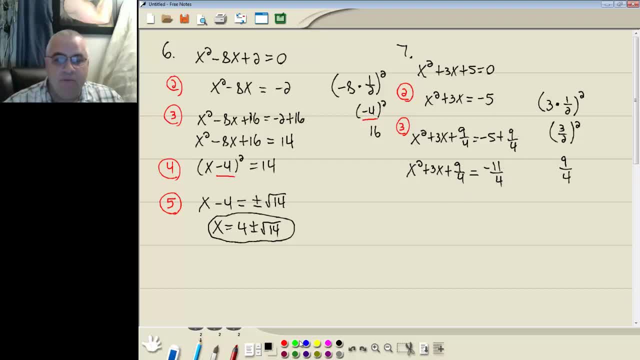 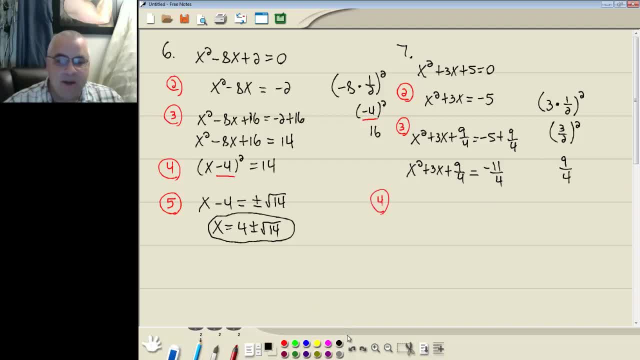 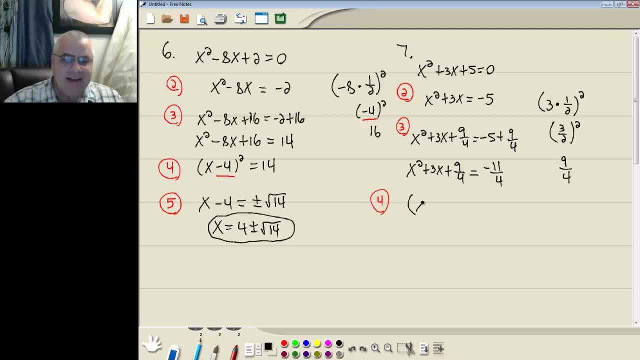 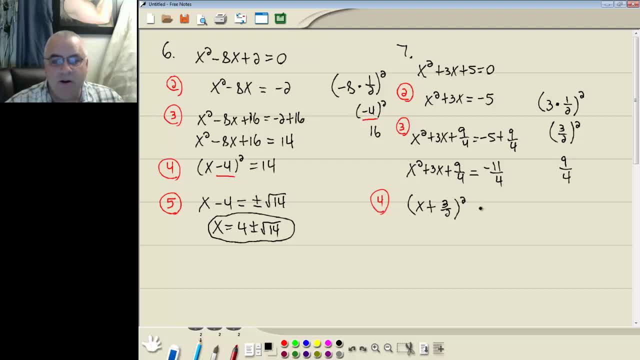 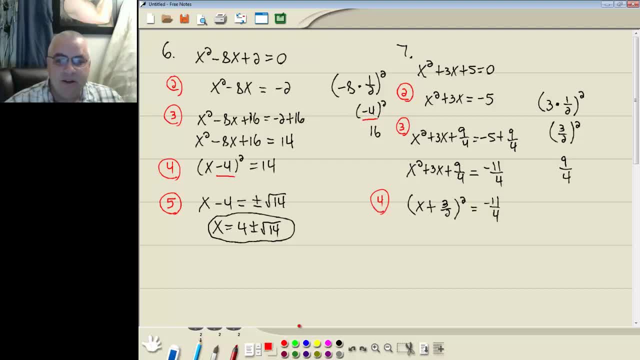 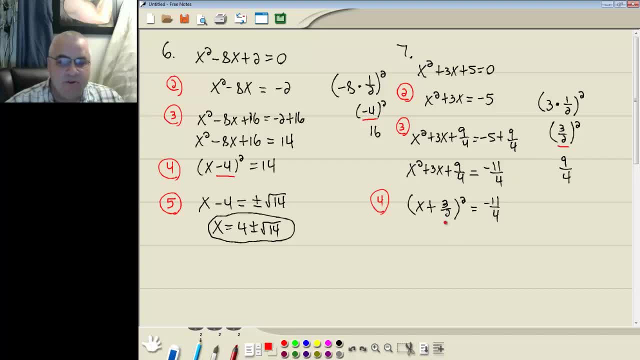 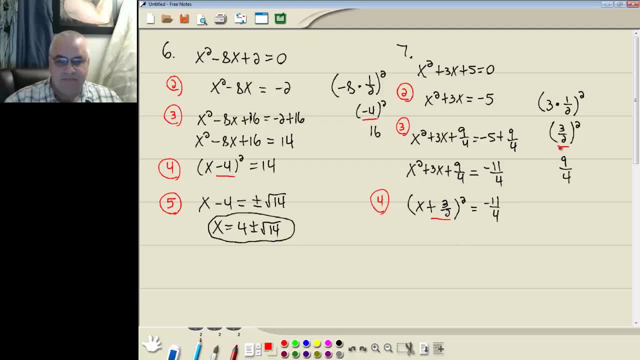 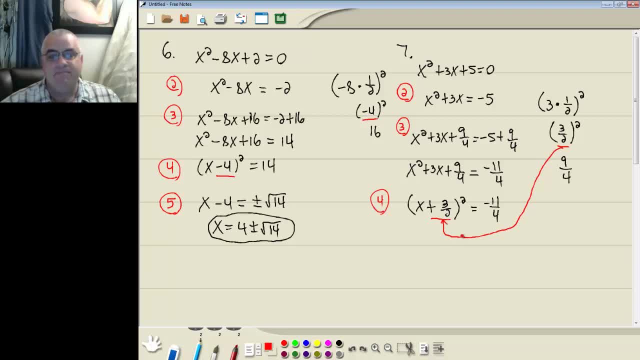 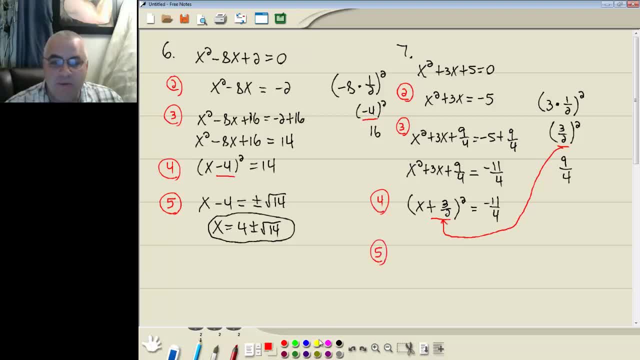 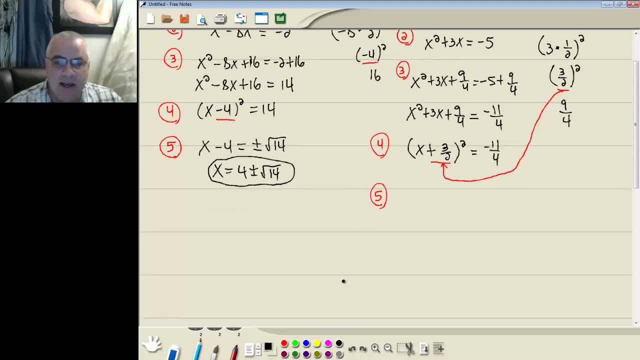 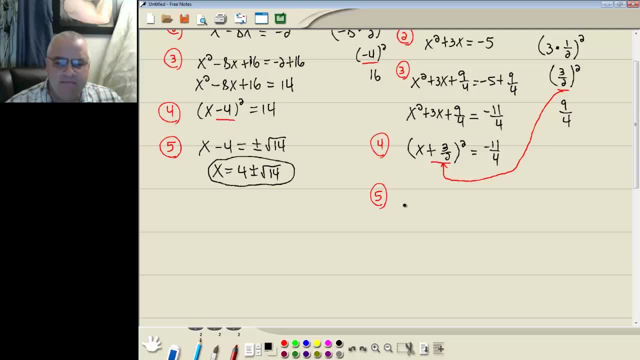 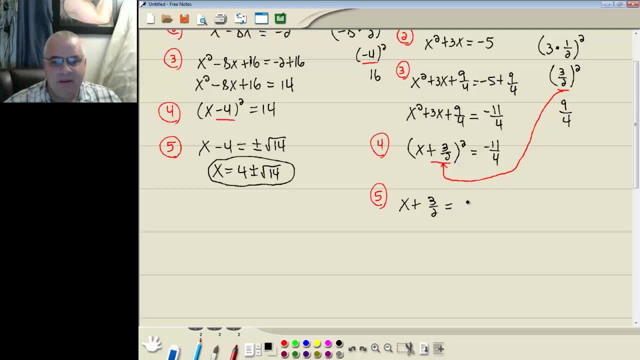 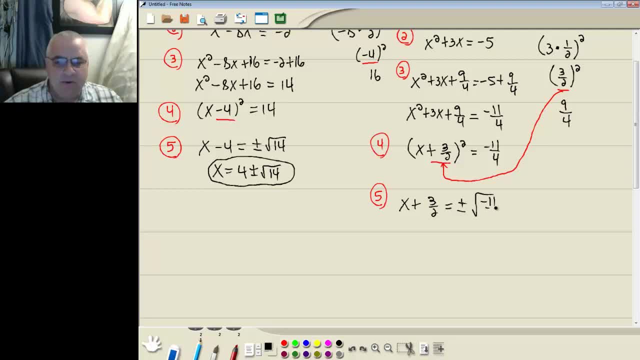 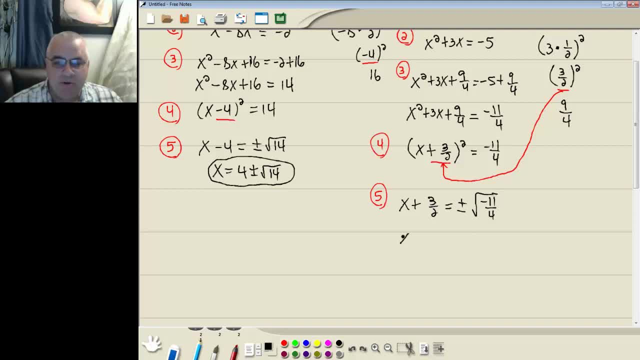 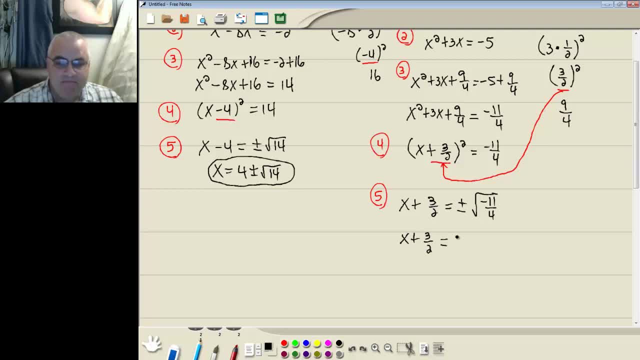 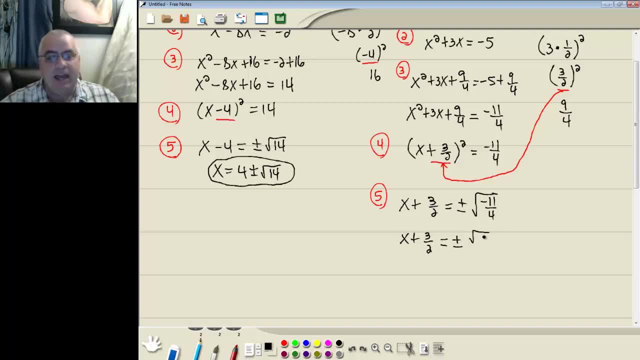 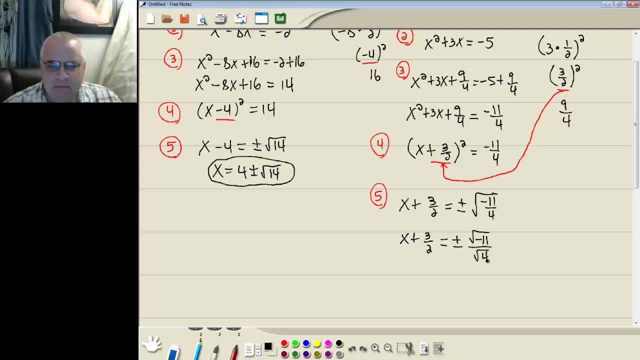 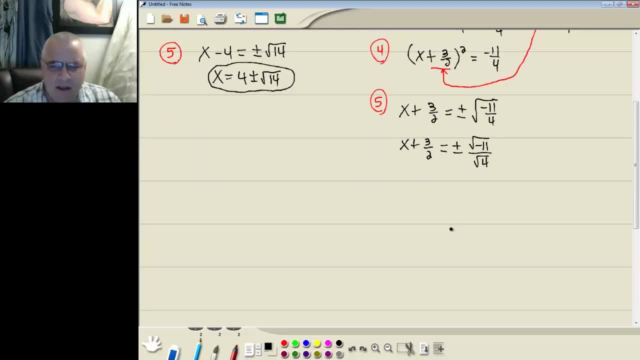 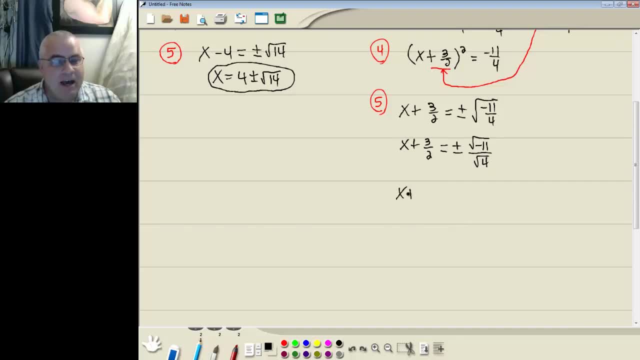 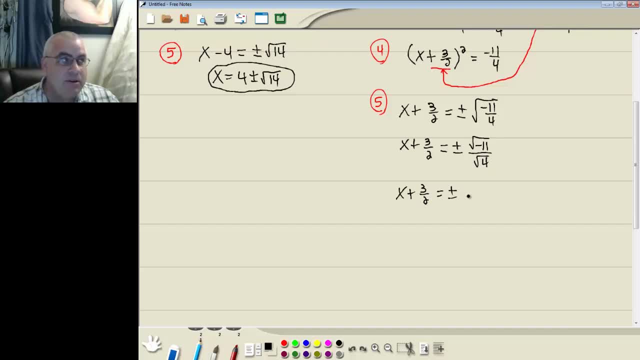 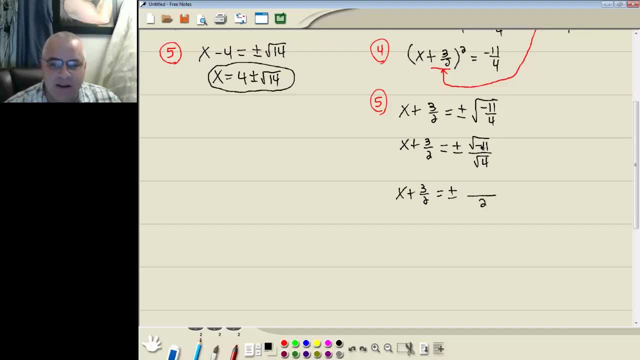 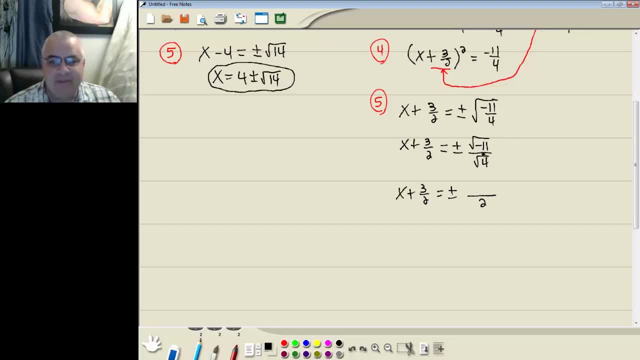 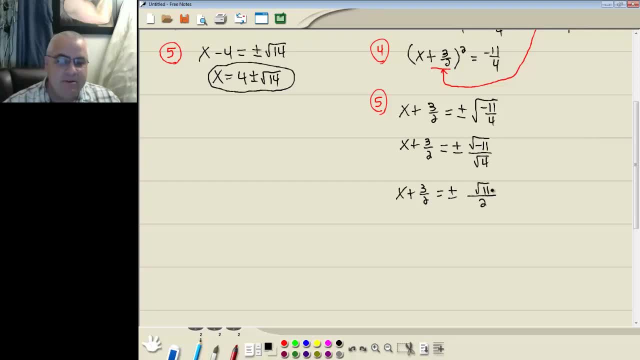 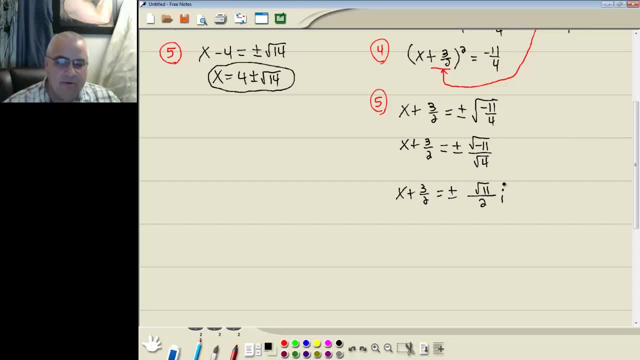 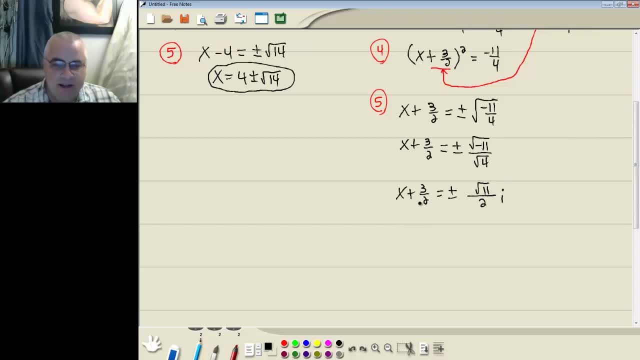 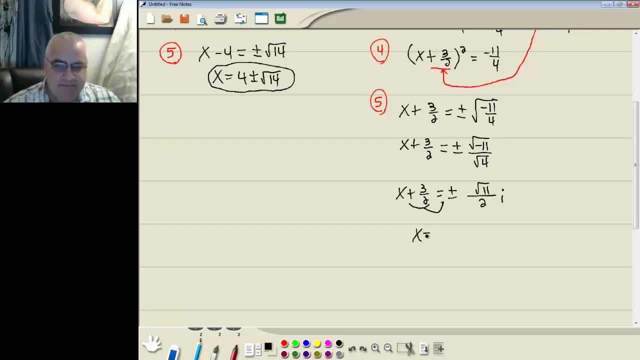 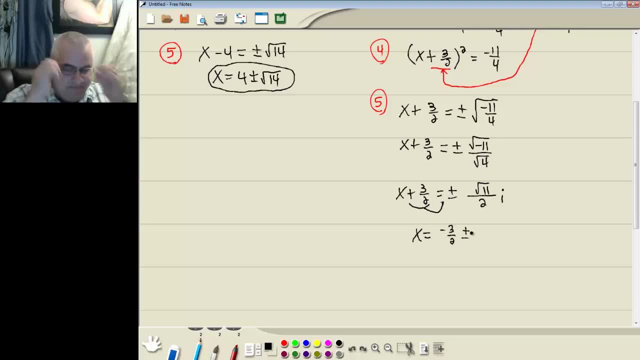 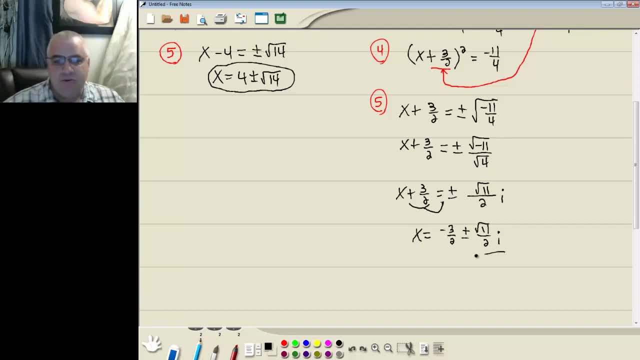 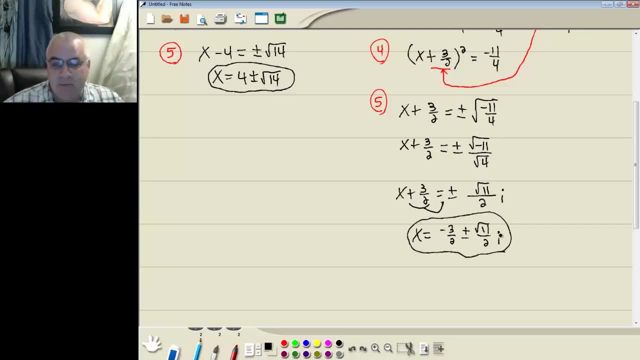 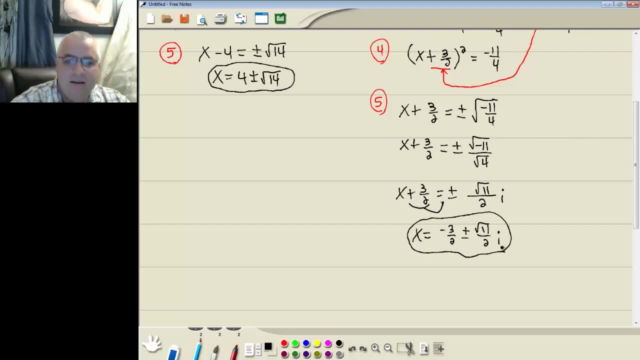 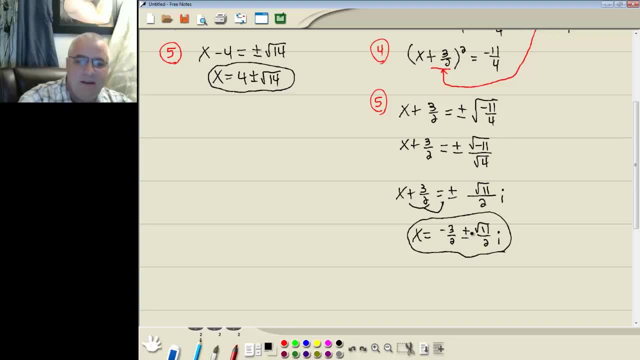 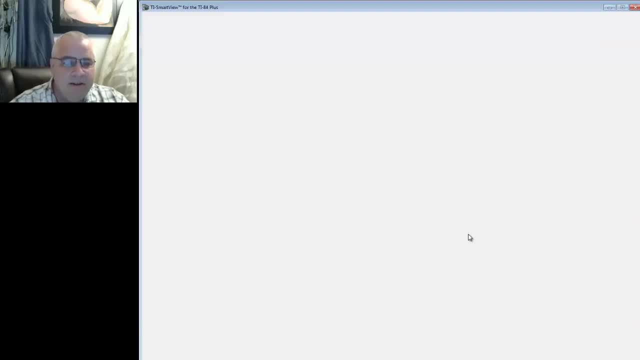 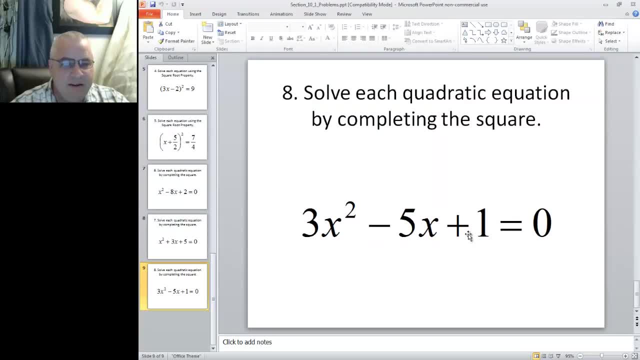 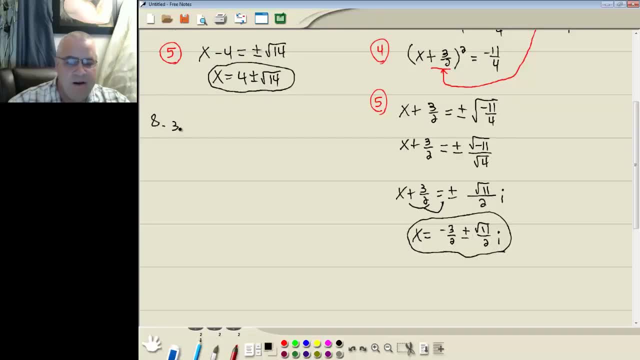 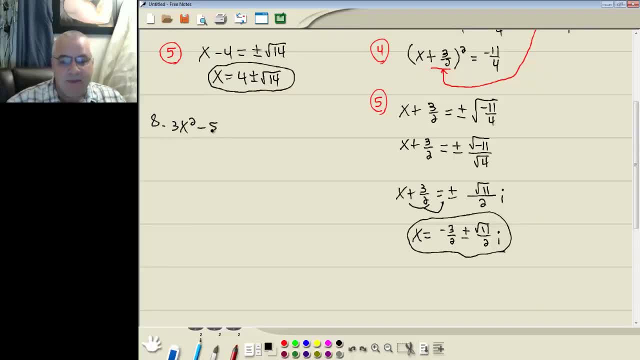 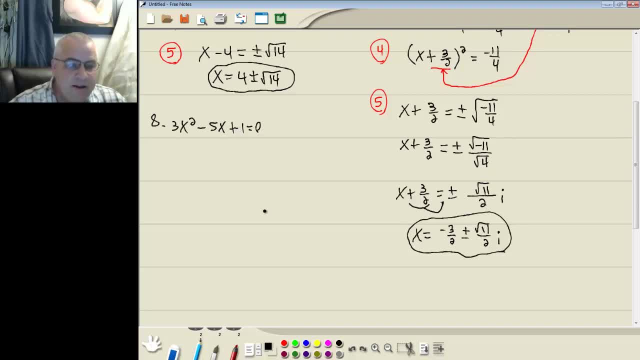 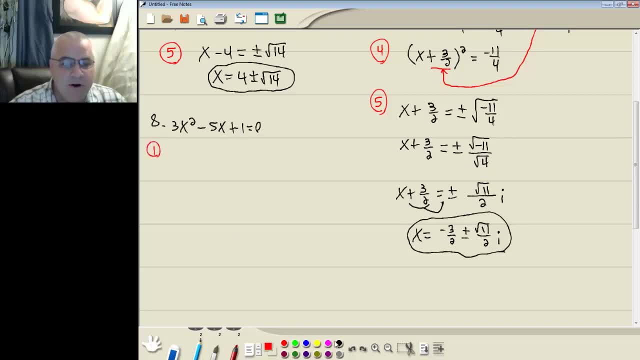 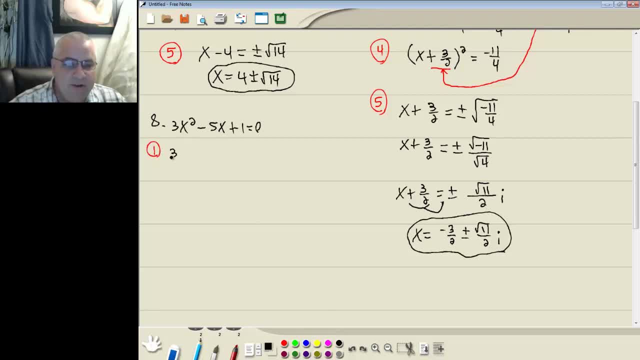 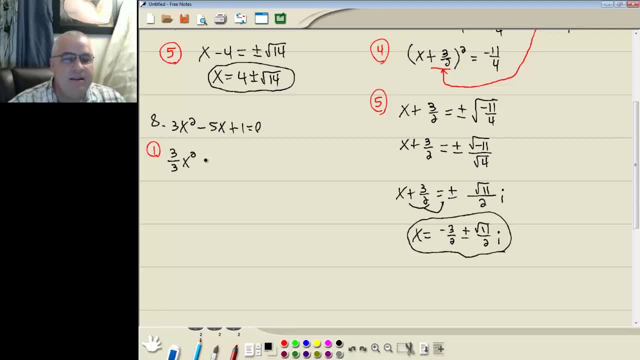 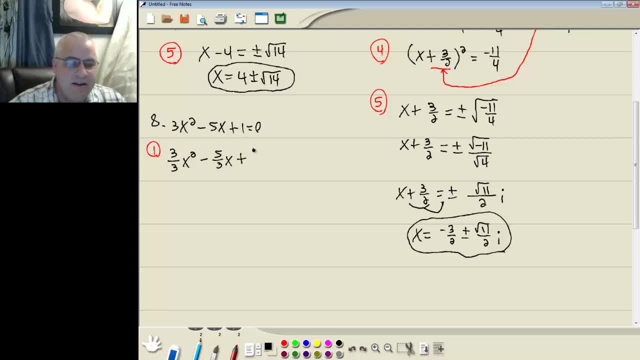 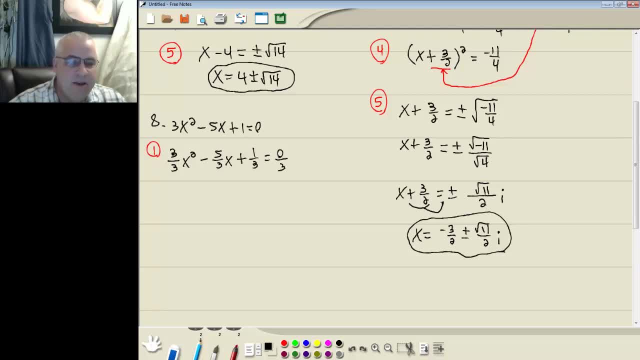 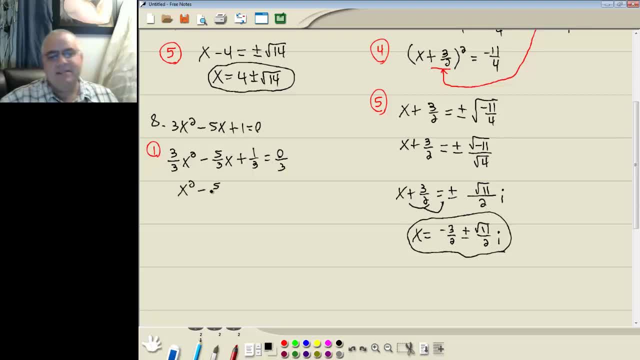 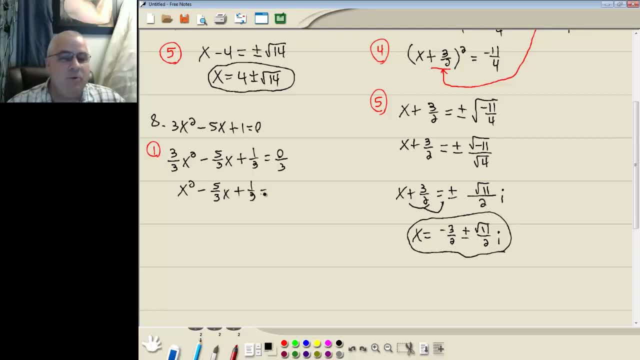 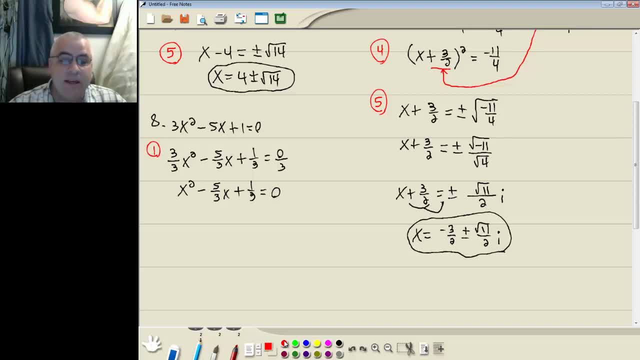 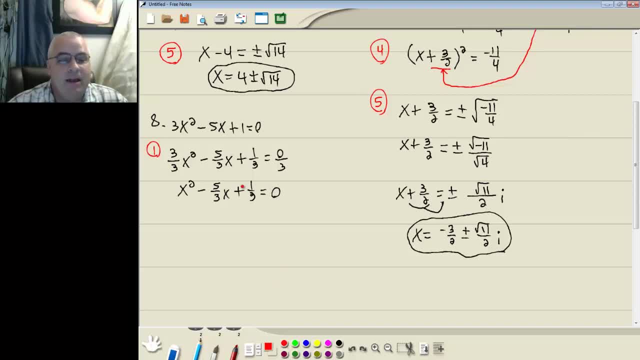 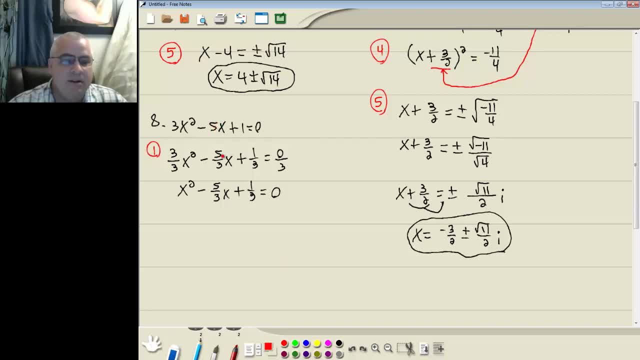 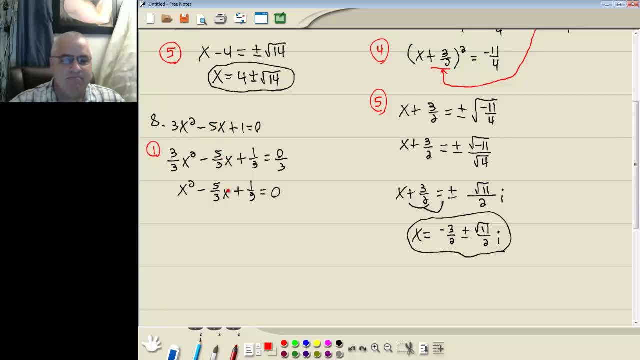 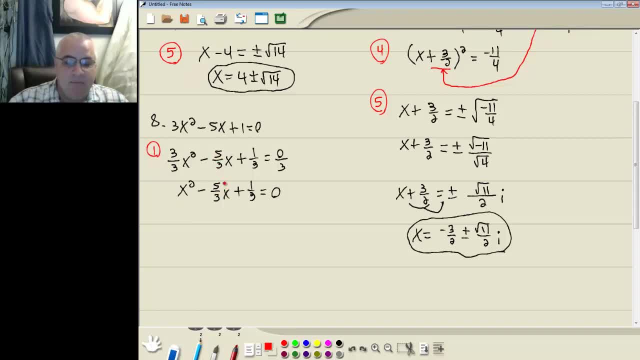 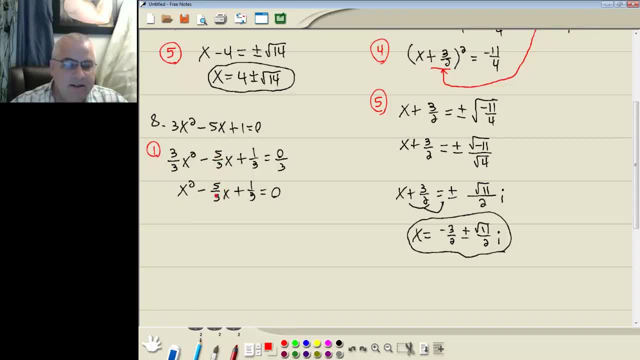 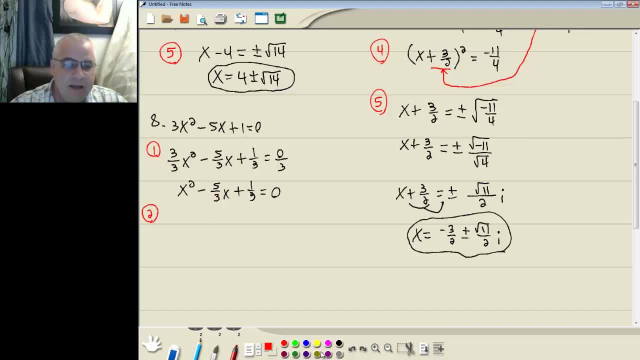 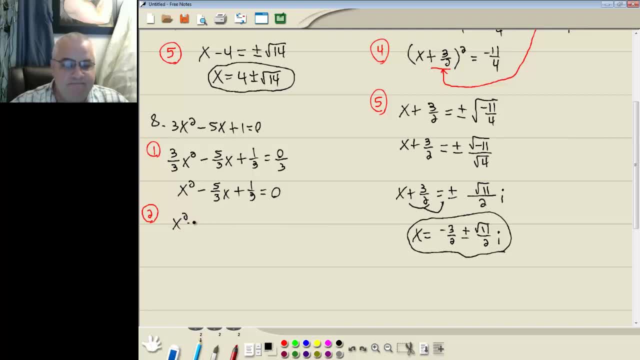 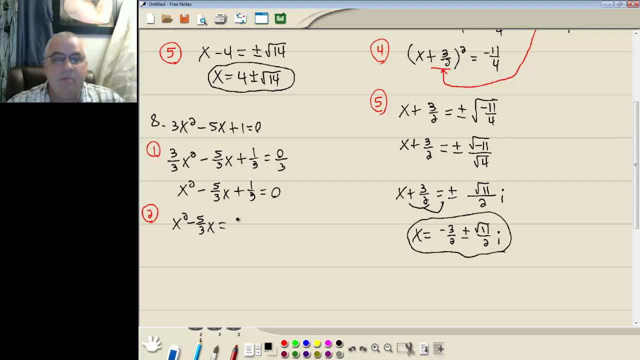 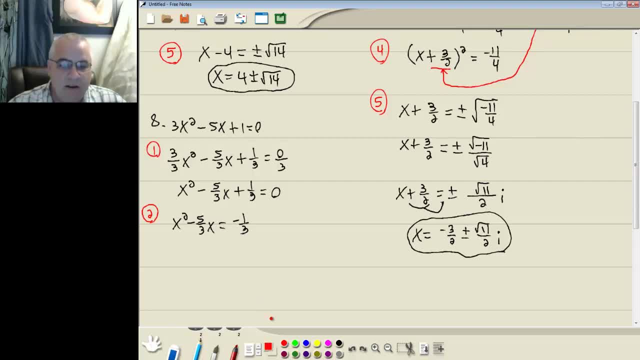 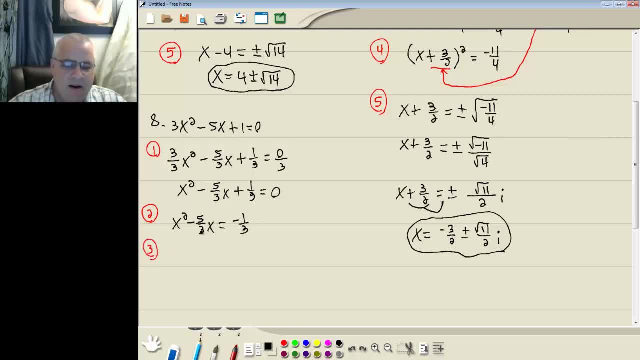 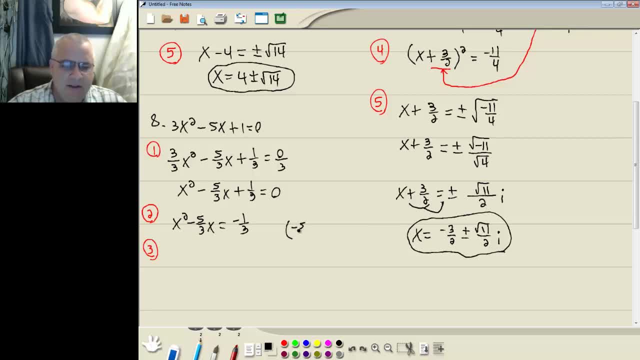 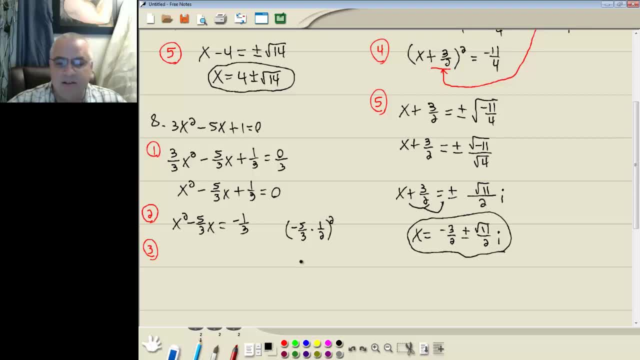 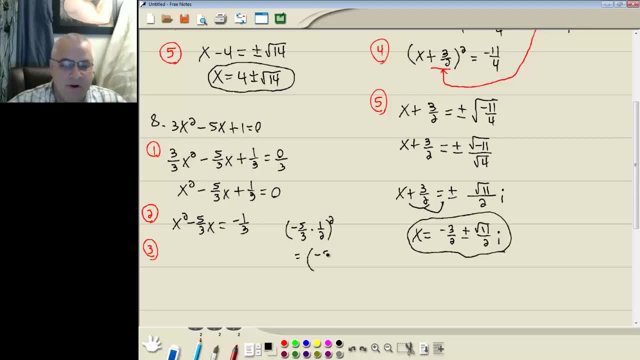 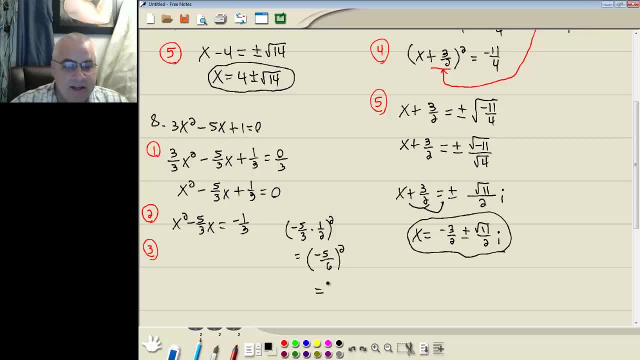 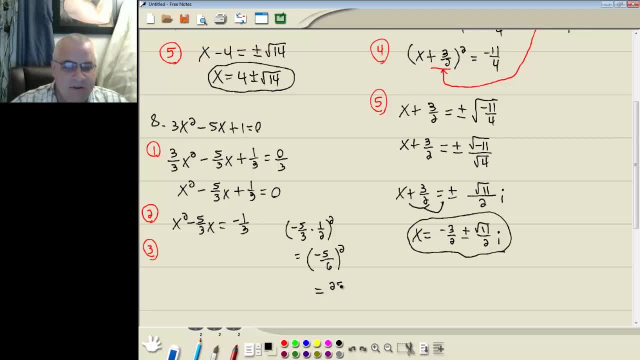 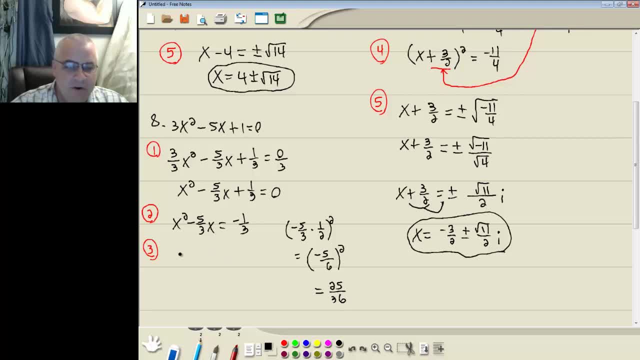 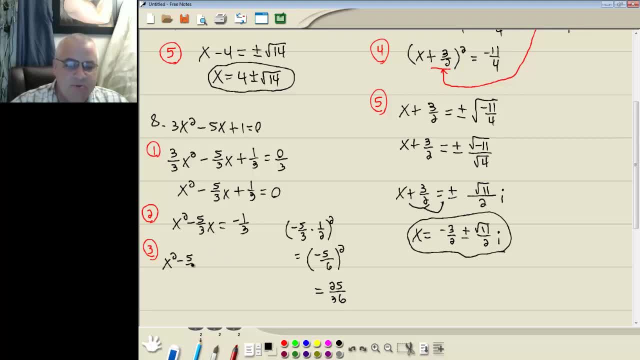 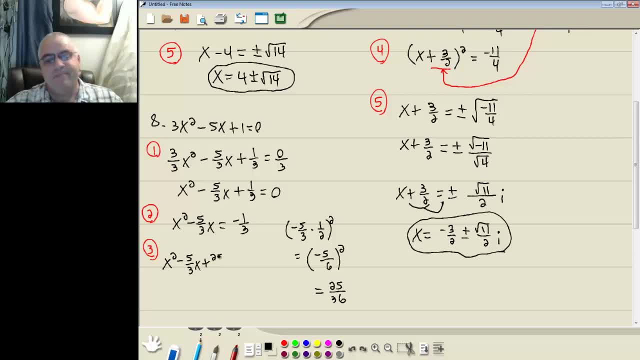 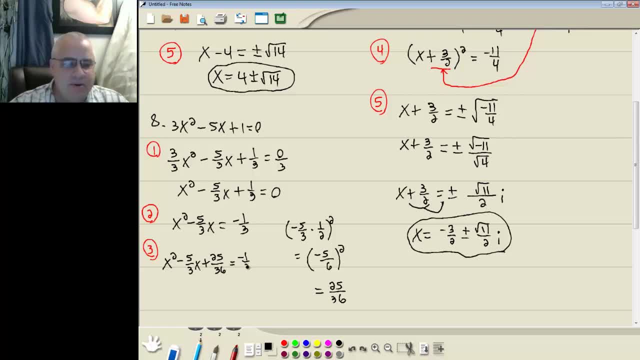 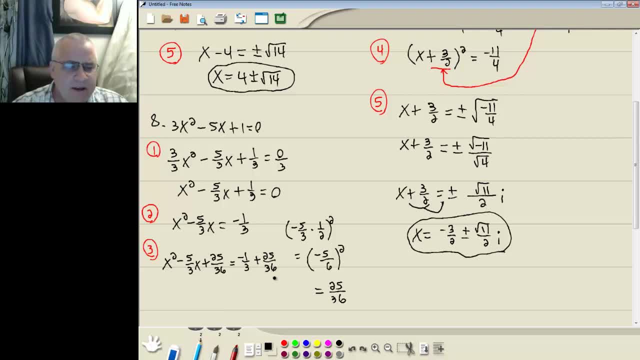 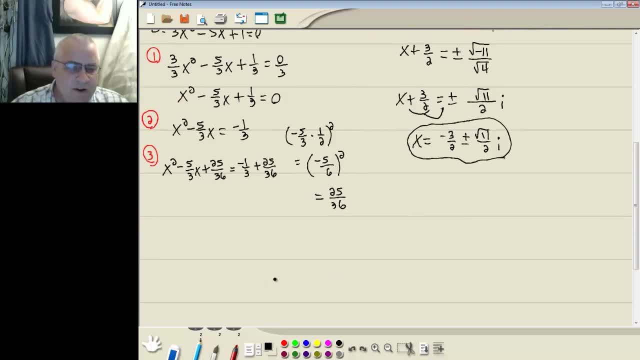 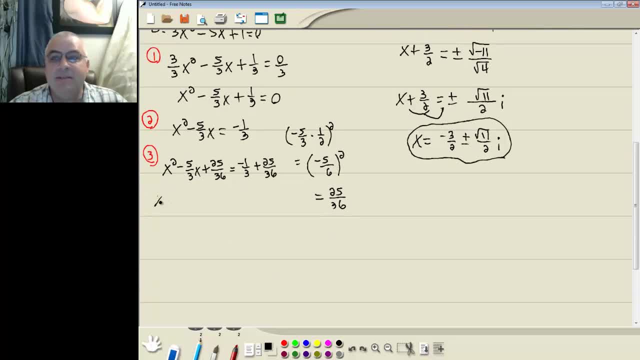 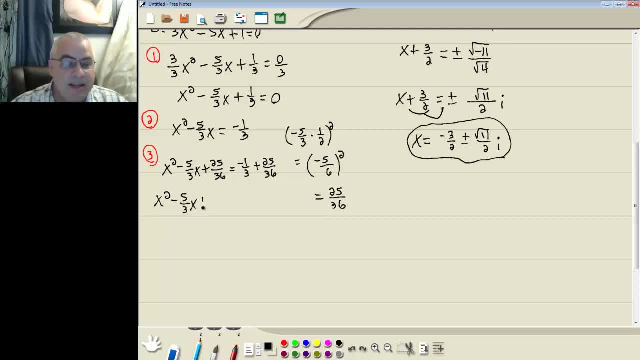 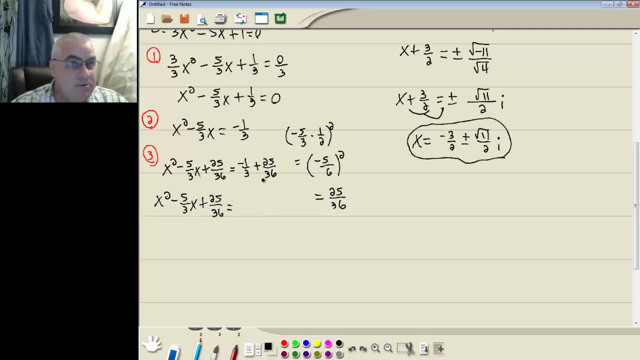 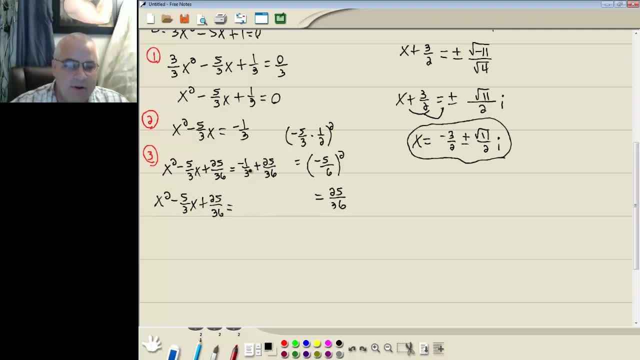 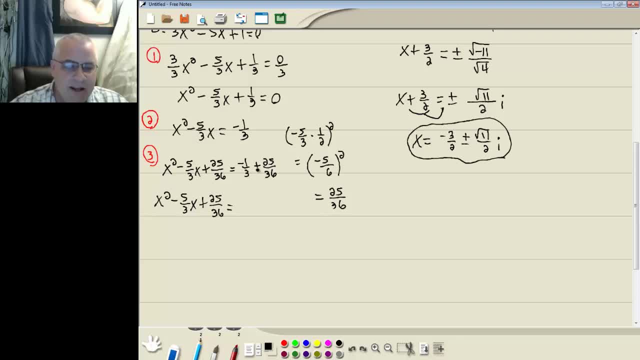 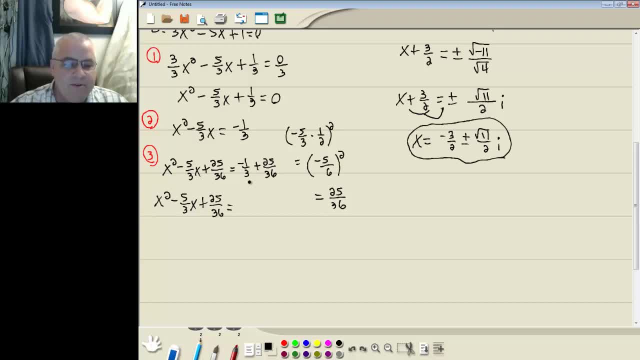 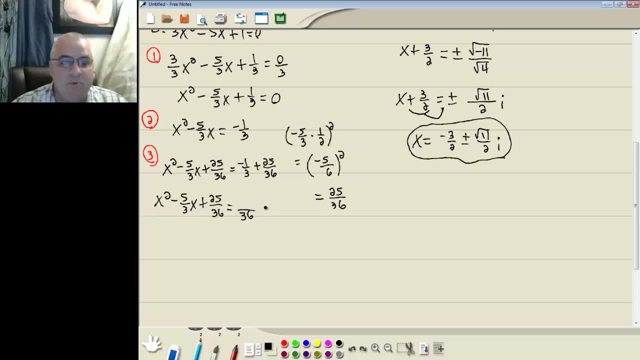 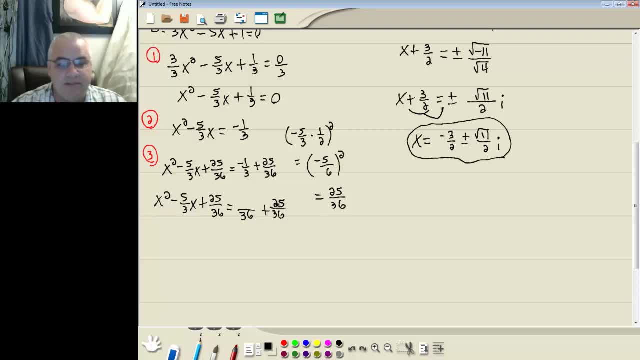 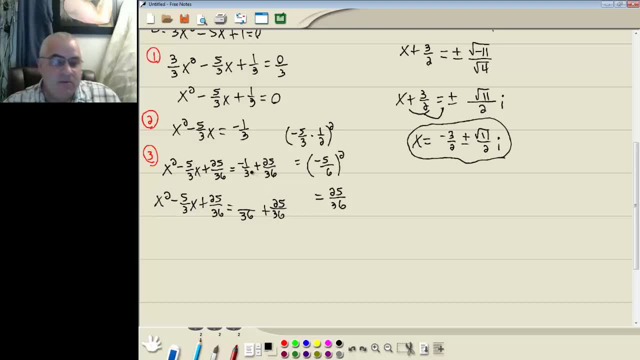 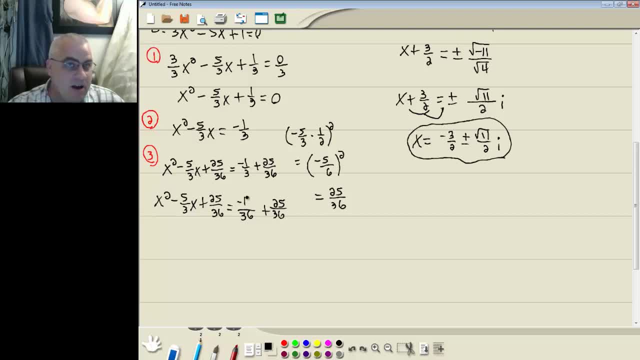 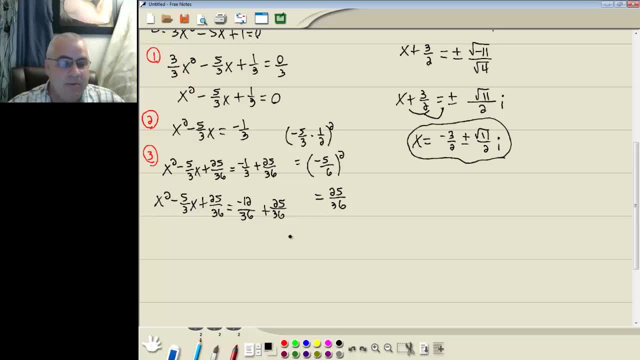 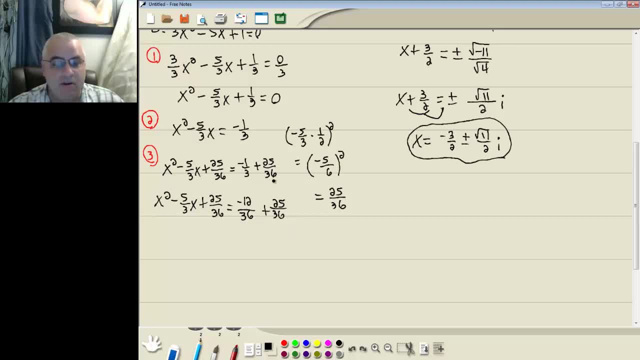 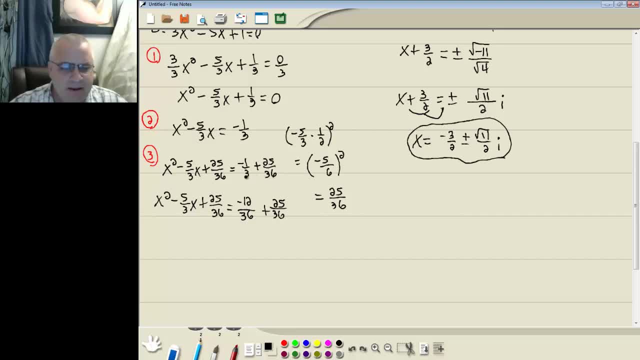 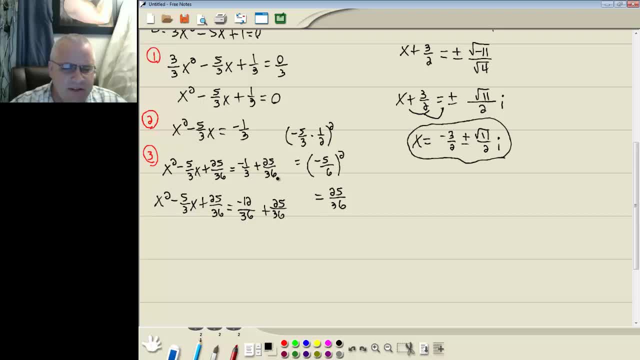 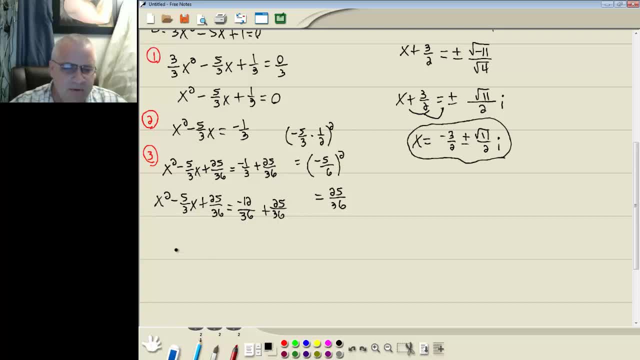 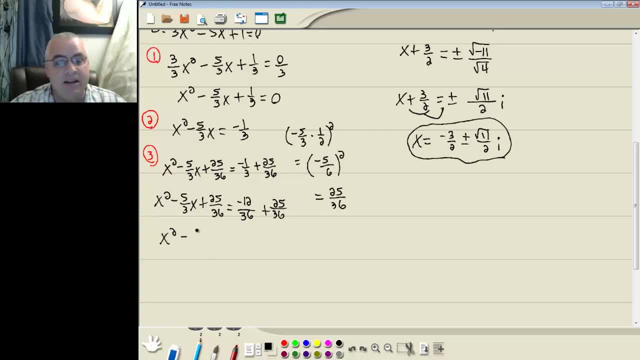 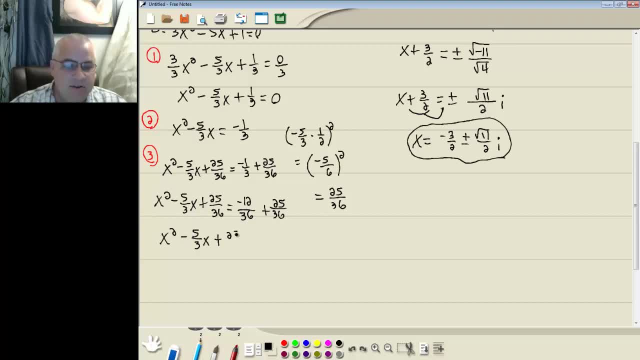 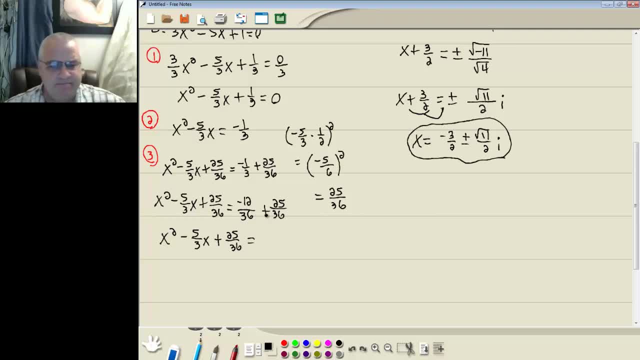 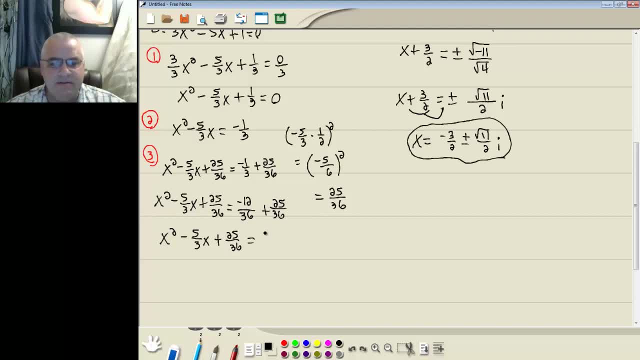 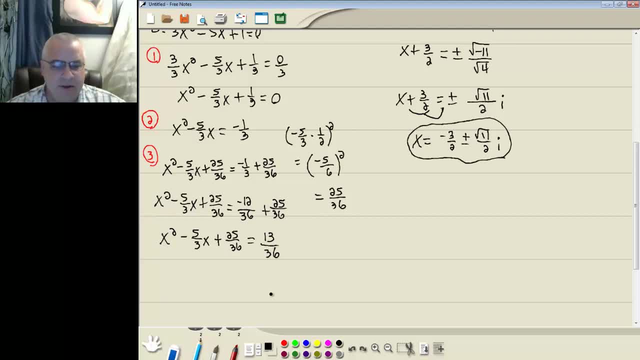 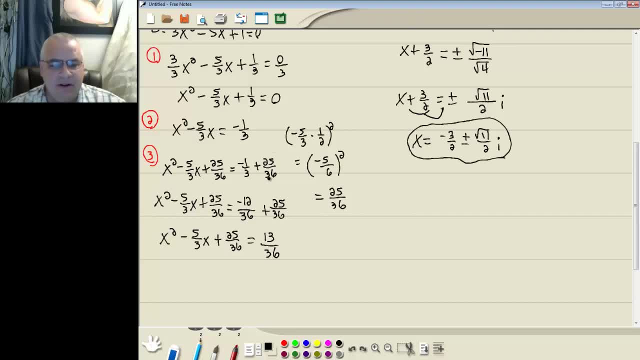 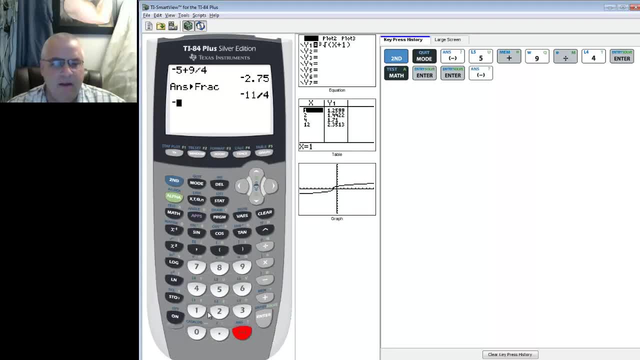 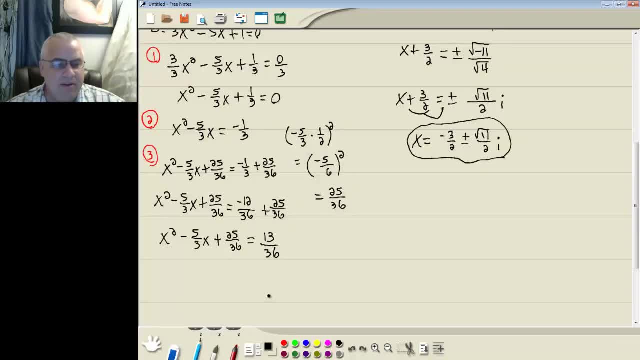 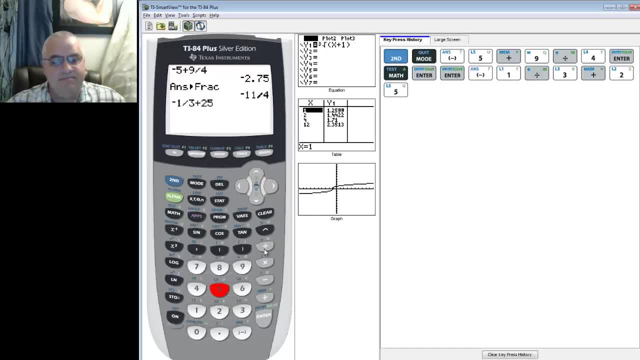 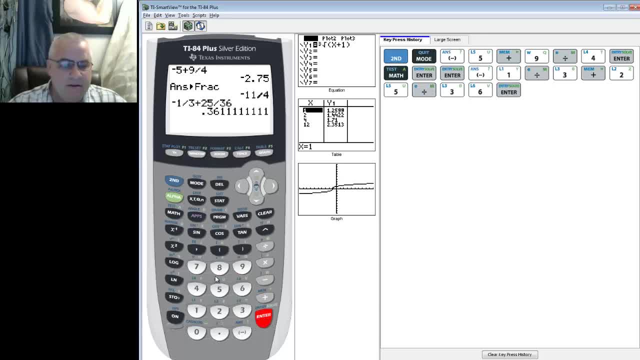 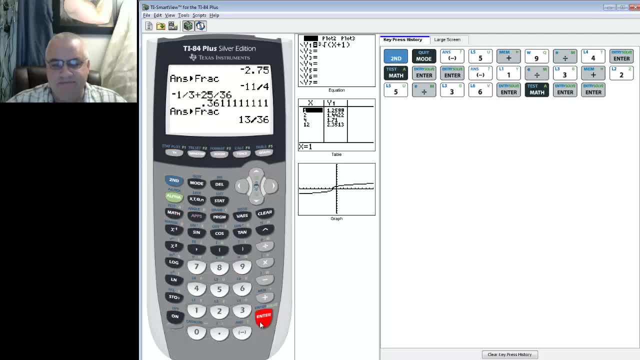 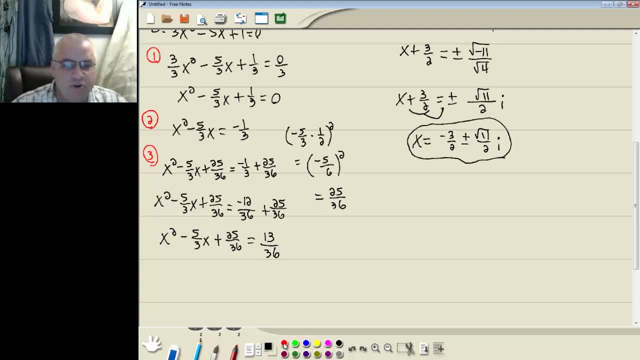 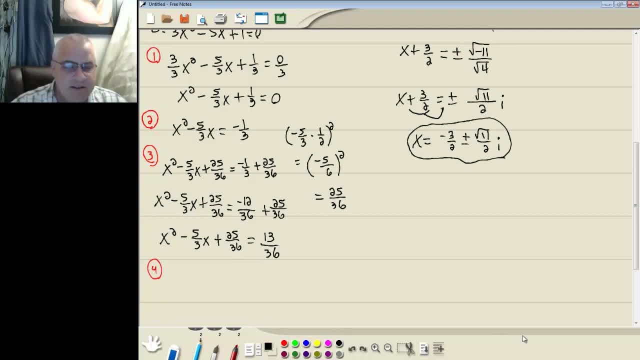 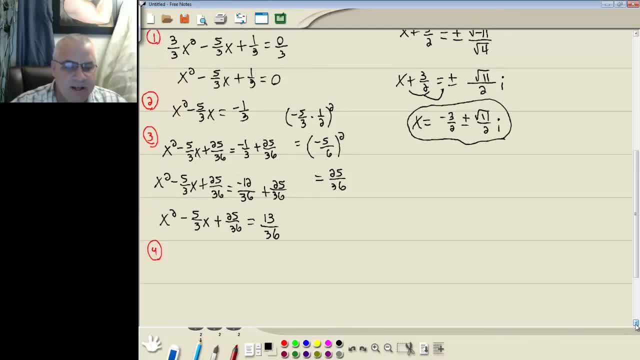 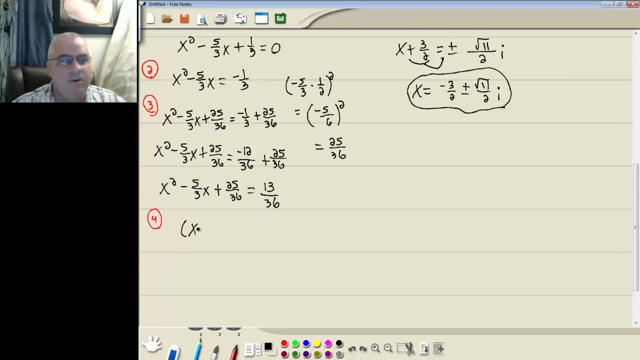 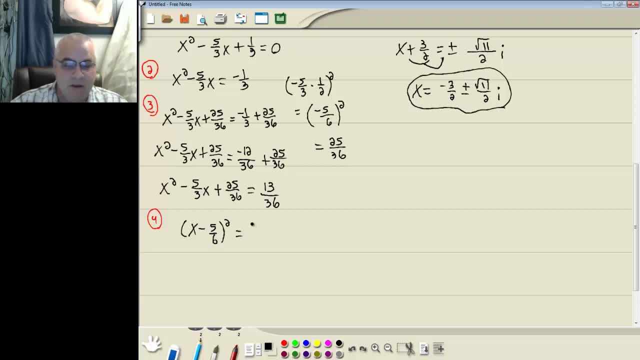 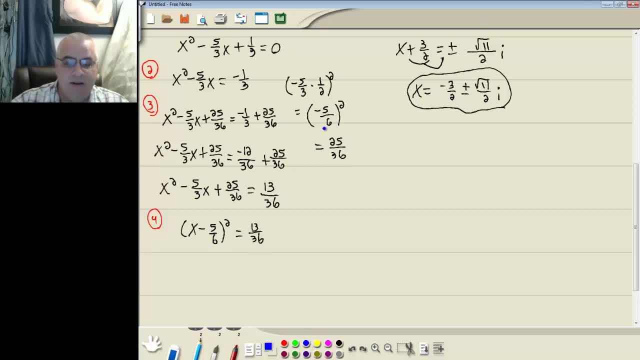 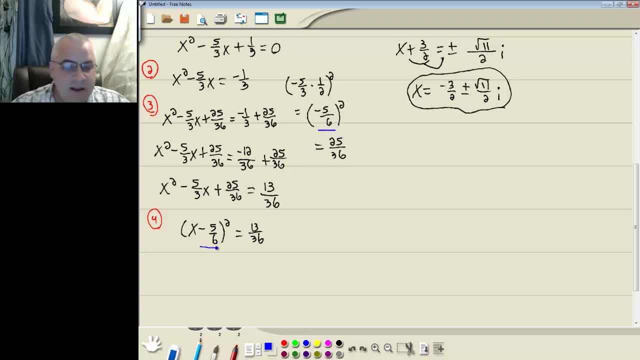 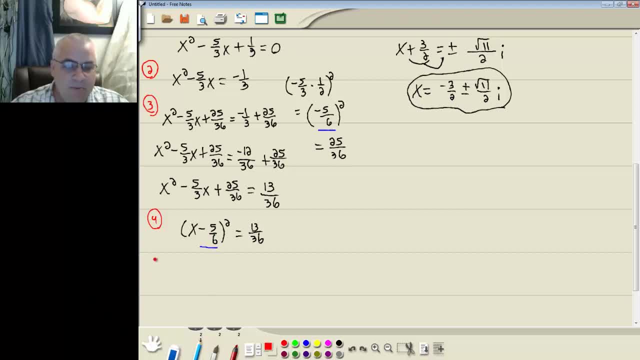 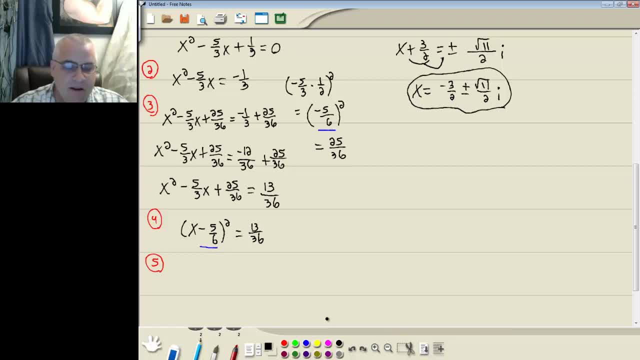 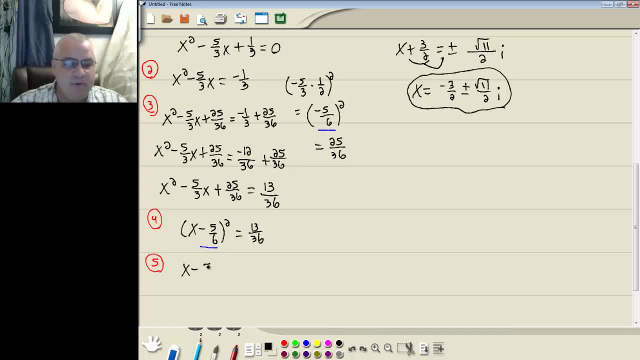 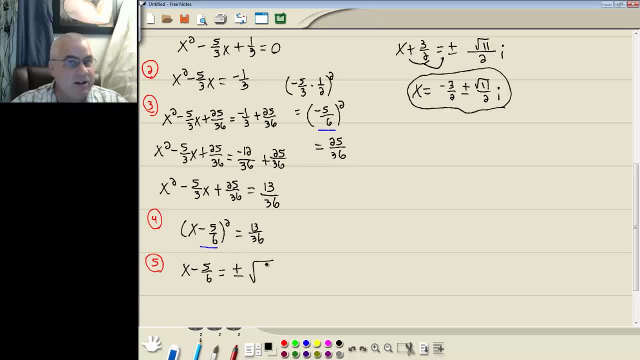 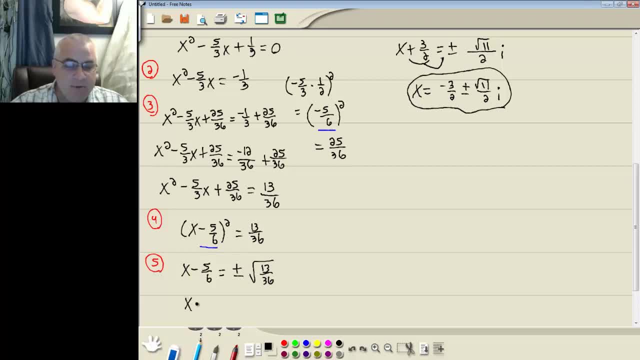